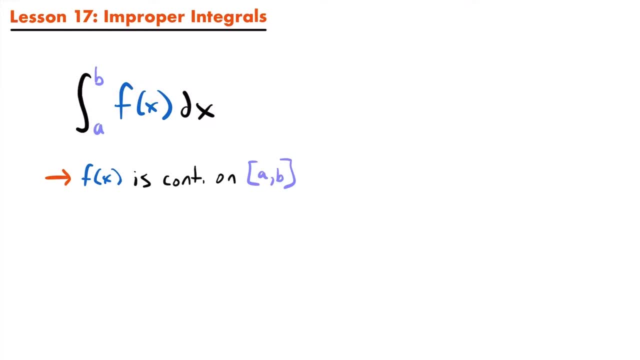 we have a definite integral from A to B of some function f of x. we have only been solving integrals where that function f of x is continuous on the closed interval from A to B. That means our function is continuous for all values between A and B and including A and B as well, And so for 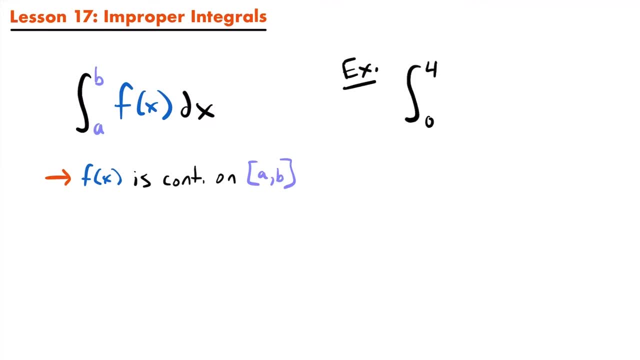 example, if we have the integral from zero to four of x squared dx and we wanted to solve this integral, note that x squared would be our function f of x and x squared is continuous for all the values from zero to four, including zero and four right. So we would say that x squared 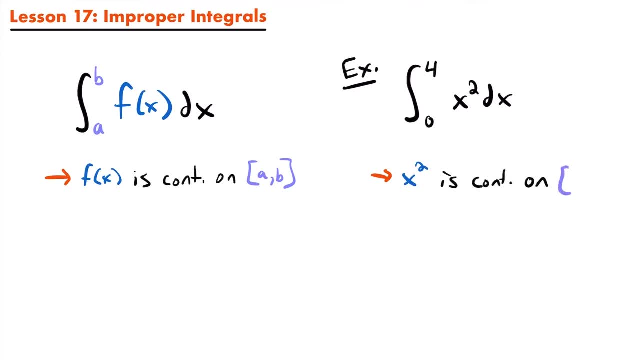 is continuous on the closed interval from zero to four. Alright, and so these are the types of integrals we have been working with so far. In fact, the continuity of the function for the range of values between your bounds or limits of integration is required by the definition of a definite integral as well. 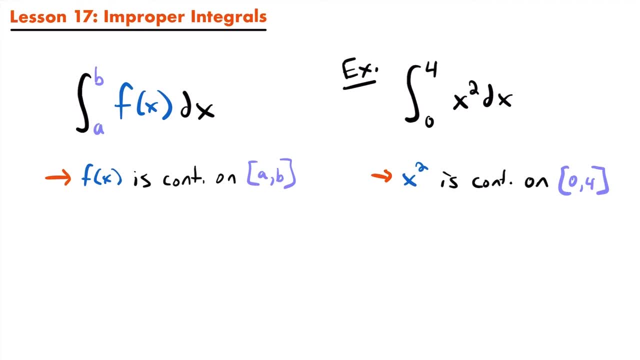 as the fundamental theorem of calculus. However, we are now going to look at how to evaluate definite integrals where the continuity requirement is not met, And these types of integrals are what we call improper integrals. And so there are two reasons that an integral will be an improper. 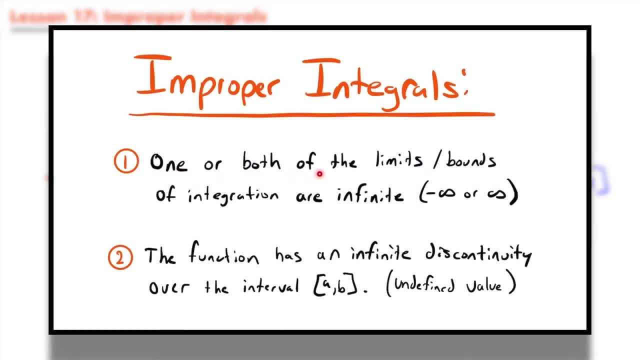 integral. The first reason is if one or both of the limits or bounds of integration are infinite, and so that would be negative infinity or infinity. So if you have a definite integral where the lower bound is zero but the upper bound is infinity, then you have an improper integral. 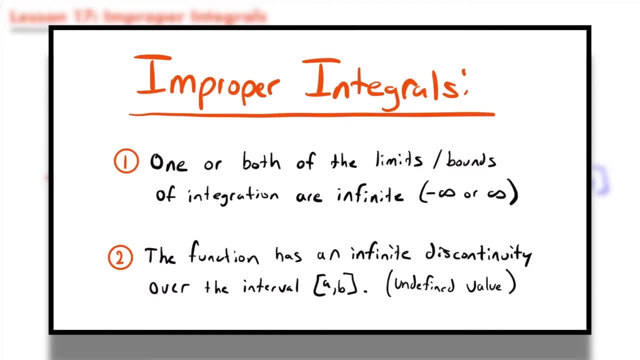 because one of your bounds is infinite. The second reason that you could have an improper integral is because the function you're integrating is the way thattırum of 8 becomes a done function. This king of sign tie will not have something without the lower bound, the bottom boundary and the expanding interval. 어떡ung swe pi $u. 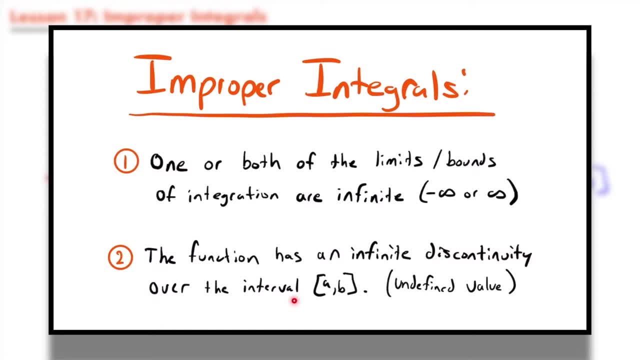 has an infinite discontinuity over the interval that you are integrating it over. Essentially, what that means is that there is an undefined value for that function somewhere on that closed interval from a to b. Another way to think about this is that the limit from either side of the function 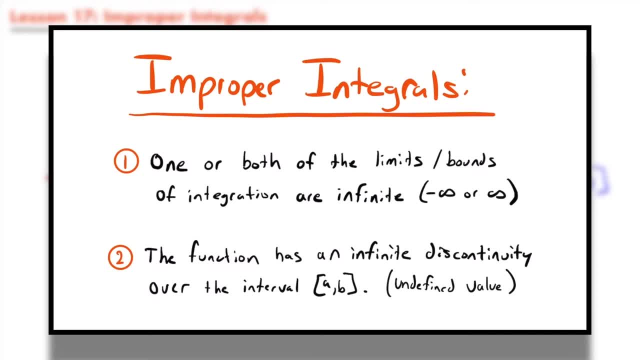 at that point of discontinuity will be infinity or negative infinity, And so that's why it's called an infinite discontinuity. But essentially, if you boil it down to the simplest definition, just know that you have an improper integral if the function you want to integrate. 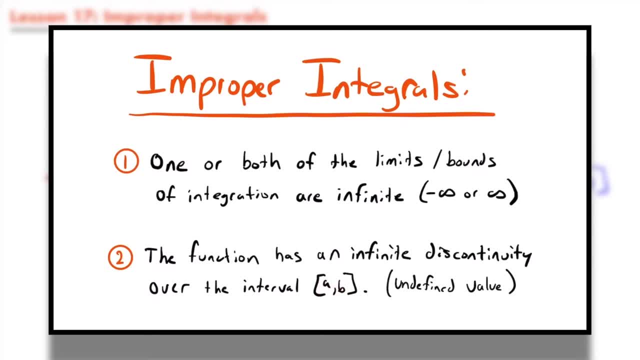 is undefined at a value between the bounds of integration or an undefined value at one of those bounds of integration. Now we're going to look at examples of improper integrals that have one of these two properties. but we're going to start by looking at improper integrals where at least one of the bounds 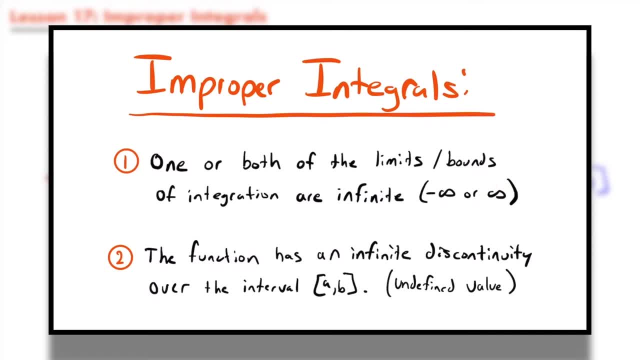 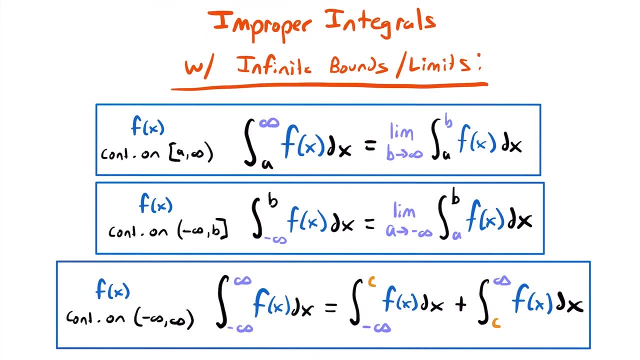 are infinite, meaning that they are negative infinity or positive infinity. All right, so first we're going to look at how to handle improper integrals. We're going to look at integrals that have infinite bounds or, if you like to call them limits, infinite limits. 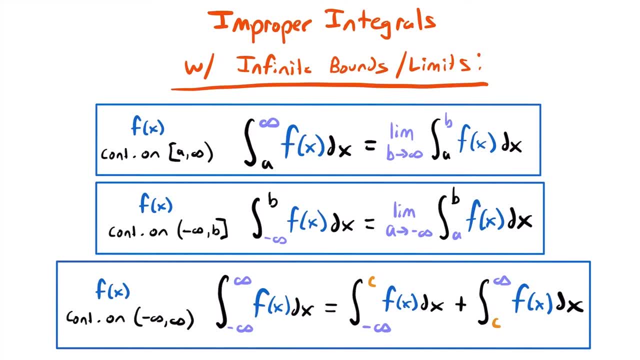 Now, in both cases, for both types of improper integrals, the way we're going to deal with them is by introducing a limit, But how we use that limit is going to differ just a little bit for each type, And so first we're looking at integrals that have an infinite bound. 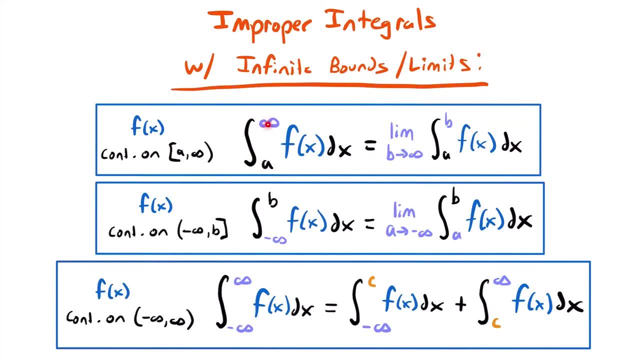 And so first up here we have an integral from a to infinity of f, of x, dx. If you have an integral like this, where you're integrating some function from some lower finite bound to an infinite bound, what you want to do is rewrite that. 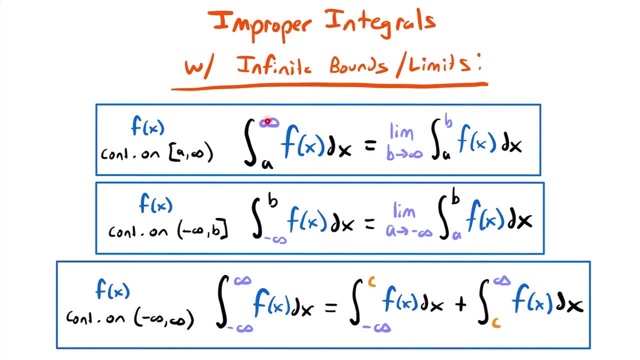 integral by replacing infinity, your infinite bound, with b, and then you want to take the limit of that integral as b approaches infinity, And then you will evaluate the definite integral as usual, but then your evaluation is going to have b in it, and so then you will take the limit, as b approaches infinity, of that. 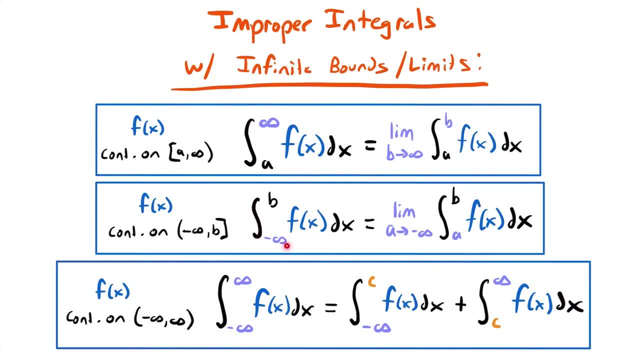 evaluation. All right. but then if you have the integral from negative infinity to infinity, you're integrating from negative infinity to b, where the upper bound is finite and the lower bound is infinite. then once again, you want to rewrite your integral by replacing negative infinity. 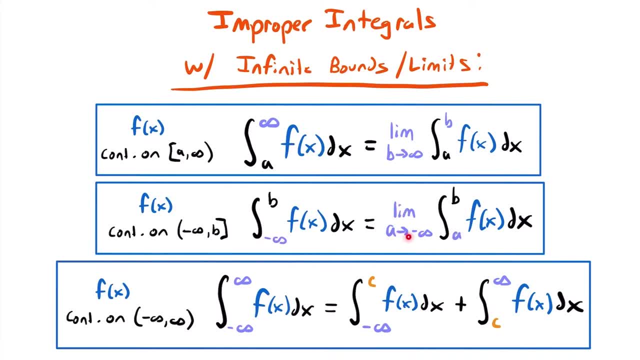 with a, and then you want to take the limit as a approaches negative infinity for that integral, All right. and then, finally, if you have an integral where both bounds are infinite, you are integrating from negative infinity to infinity. then what you want to do is choose. 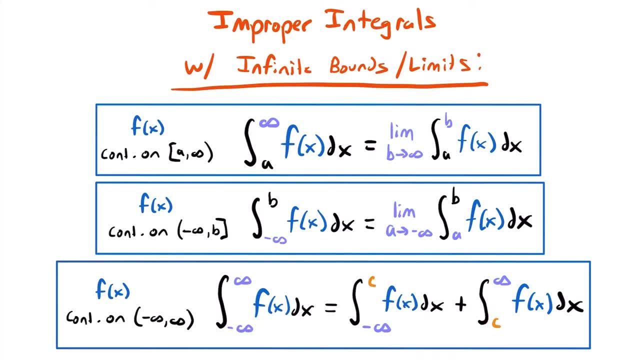 some convenient value c, that is between negative infinity and infinity. And you will break up that integral into two integrals where you have negative infinity to that value of c for the first integral and then the second integral. you integrate from c to positive infinity. 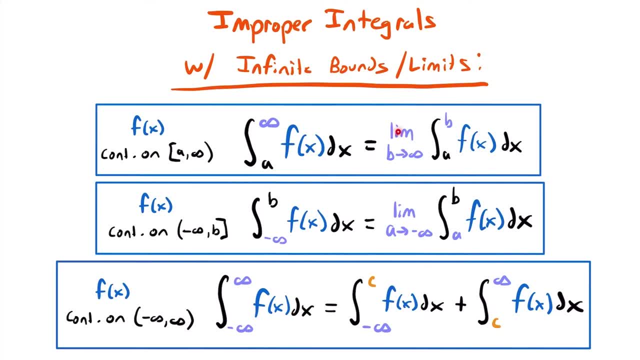 And then you would rewrite each of these integrals with the limits above Right, so we would change negative infinity to be a and then take the limit of this integral as a approaches negative infinity. And we would do the same thing for this integral, but set infinity equal to b. and then we would 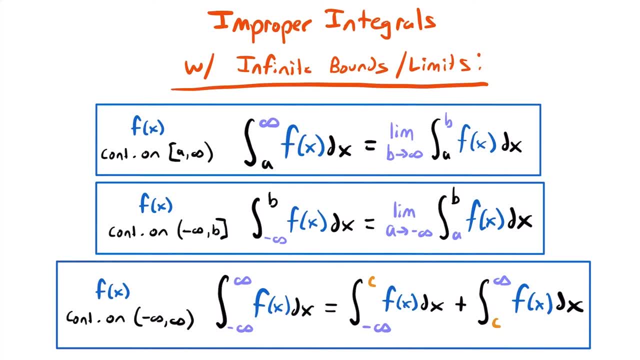 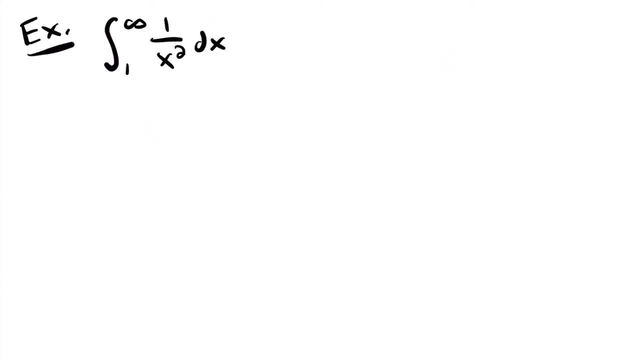 take the limit as b approaches infinity. All right, so that might be a lot to soak in at first, but it's actually not as complicated as it looks, and you'll see that as we look at our first example. All right, so here's our first example. 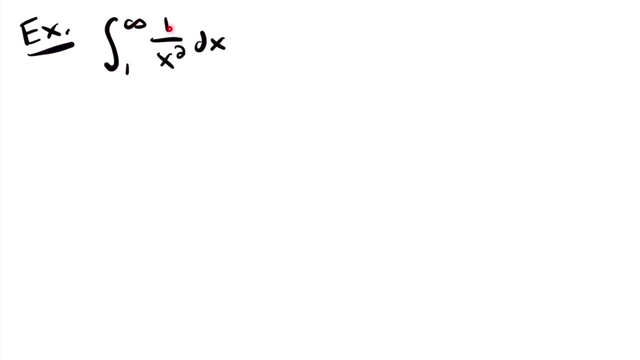 We have the integral from 1 to infinity of 1 divided by x squared dx. Now this is clearly an improper integral, because our upper bound is infinity. The moment that you see that you have an infinite bound, you know you are working with an improper. 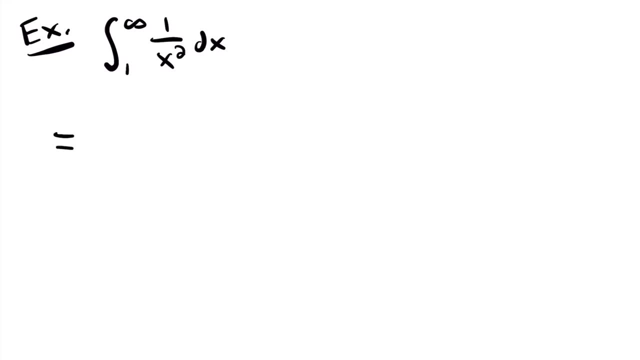 integral, And so what we want to do is rewrite this integral using a limit. We are going to replace infinity with b and then take the limit of our integral as b approaches infinity. So we're going to have the integral from 1 to b, of 1 divided by x squared dx. but then 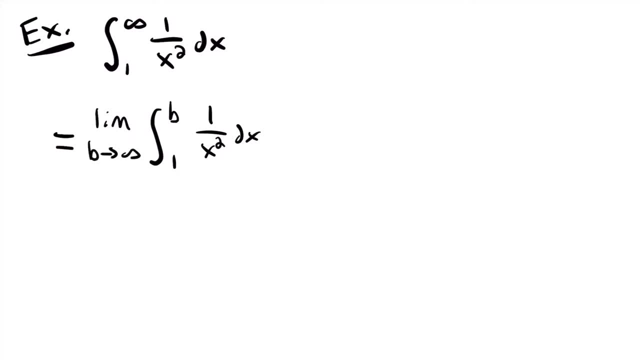 we want to take the limit as b approaches infinity. All right, so that's how we will rewrite this integral, so that we can evaluate it and then take the limit of it. to finish, our integral With the�� instructions are the following: for merged equals 2 degrees and 1 divided. 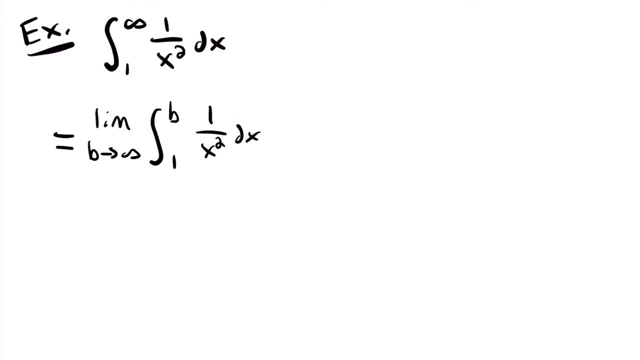 by 2 degrees and 1 divided by 2 degrees. So instead of that, we will write the derivative of the numerator and the derivative of인데요, because we do not want to be wrong founders For the first instance, maybe we should write this further: 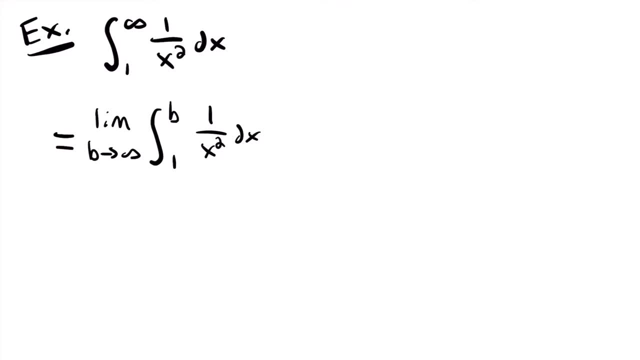 So what we can do is write the behavior of the expression, And then nearly all of the lecture, along with the expression, will come inWhereeun Bobby is presenting this, And so what happens? we do not just the general version, but we and the integral. 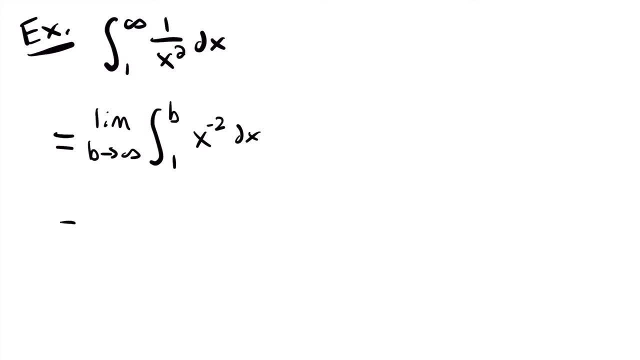 We just do not calculate the integral. We do not calculate integral equation to solve this integral. So this will be equal to the limit. as b approaches infinity of the integral of x to the negative second power, We'll add one to the exponent and divide. 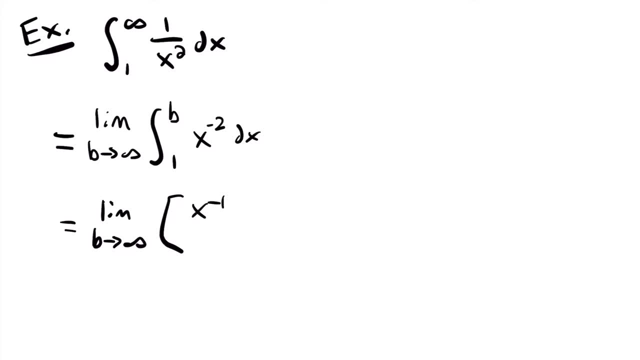 by that new exponent. So we'll have x to the negative first power divided by negative one, and that is evaluated from one to b. Now if we simplify this a little bit, we can pull that negative out front and then move x to the negative first power to the denominator. 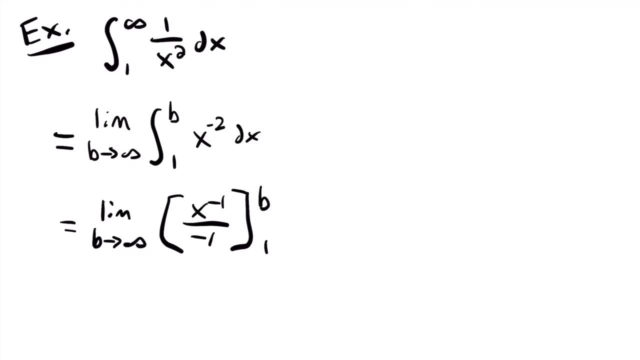 by making that exponent positive. So we'll x to the positive first power in the denominator. So this is equal to the limit as b approaches infinity of negative, one divided by x, evaluated from one to b. All right Now if we continue our work up. 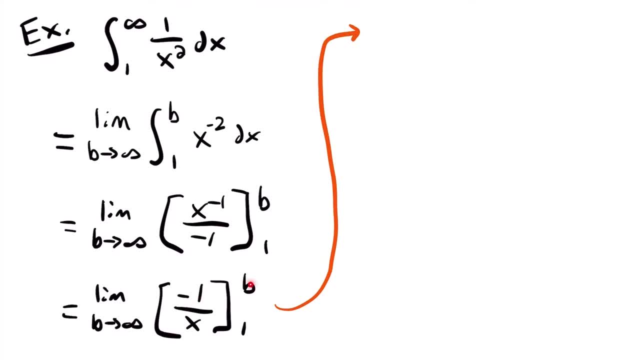 here we can now evaluate our expression at b and then subtract the evaluation at one, So we'll have that this is equal to the limit. as b approaches infinity of negative, negative one divided by x. This is, shall we freezeamos, 1 divided by b, minus negative, 1 divided by 1.. Okay, so we plugged in b for x, so we 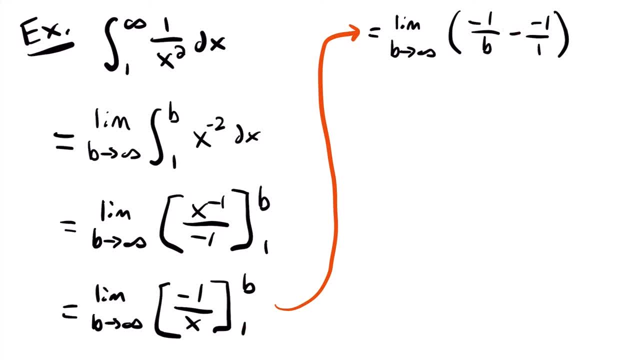 have negative 1 divided by b and then we plug in 1, so we subtract negative 1 divided by 1.. Now, if we simplify, these two negatives will cancel out, and 1 divided by 1 is 1, and so this is equal to the limit as b approaches infinity of. 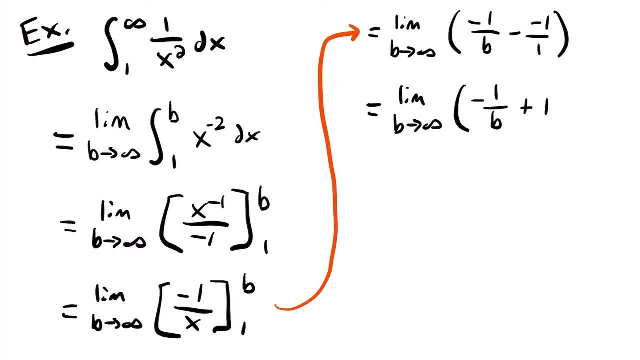 negative 1 divided by b plus 1.. Alright, now, at this point we have finished evaluating our integral from 1 to b, of x to the negative second power, but now we need to find the limit of that expression as b approaches infinity. So now we only have 1b to deal with here, and so what would happen to b as it? 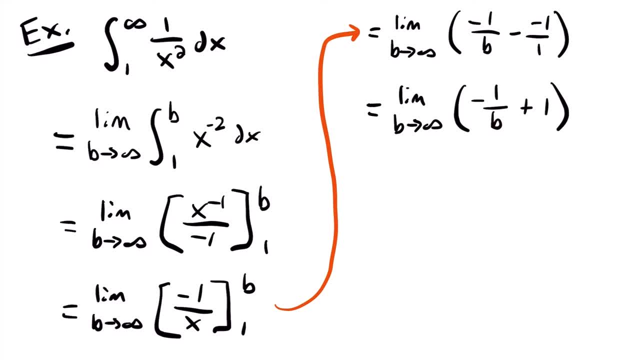 would get larger as it approaches infinity. Well, as b gets larger, the denominator of this fraction will get larger, and when you have a fixed value like 1 divided by an increasing value, that fraction is going to get smaller and smaller towards the value of 0, and so you can see this: if b 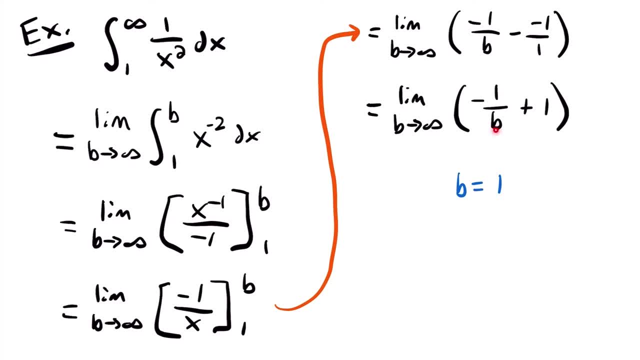 is equal to 1, then, ignoring this negative, this fraction would be 1 divided by 1, which is equal to 1.. If b is equal to 10, then we would have 1 divided by 10, which is equal to 0.1, and then, if b was equal to 100, you would have 1 divided by. 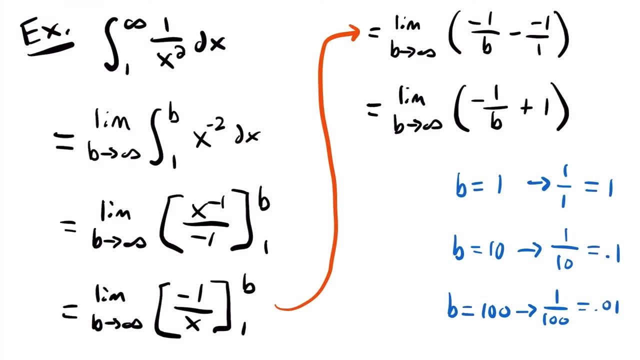 100, which is equal to 0.01, and so as you would pick larger and larger values of b, your that fraction gets smaller towards 0. And so what we can say is that 1 divided by b is equal to 0, as b approaches infinity, and then the limit of a constant like 1 is just: 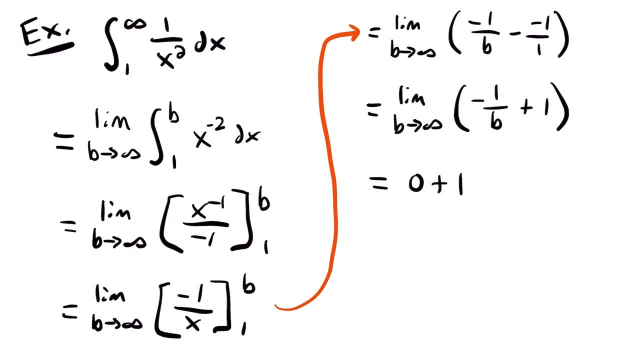 equal to that constant, and so this is equal to 0 plus 1, which is equal to 1.. And so 1 is the solution to this improper integral. Alright, now, when you solve an improper integral and you get a finite value- meaning this is not infinity or negative infinity- We say: 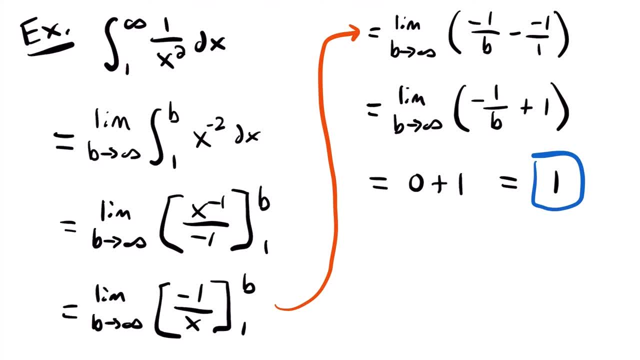 that the improper integral converges, and I'll write that out. This means that the integral converges, and all that means is that the area underneath this function, from x equals 1 to infinity, will settle at a value of 1.. It converges to 1.. 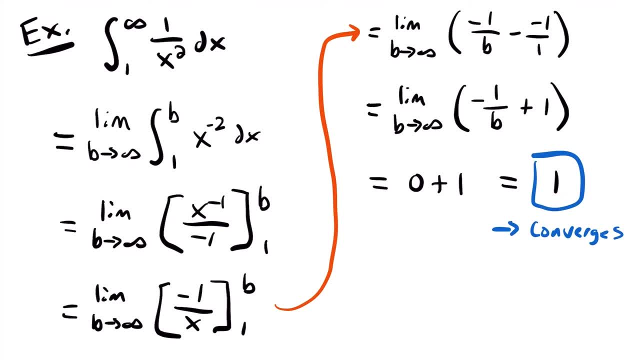 If it was not equal to 1, meaning it was infinity or negative infinity, then we would say that this forced function will reappear whenever every decimal is equal to infinity. What will you do to solve this? Easy ones, Make sure to click on the box at the top and. 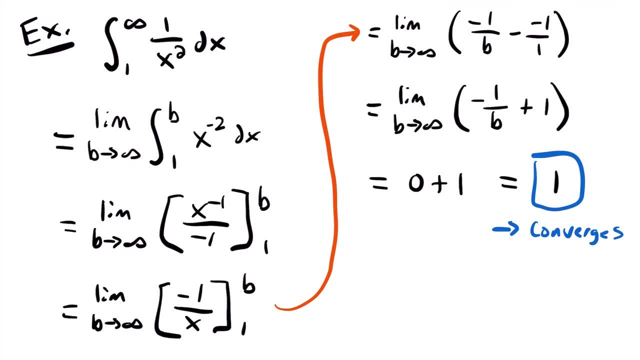 say that the improper integral diverges, meaning it does not settle at a particular value that we can express like one, Alright. and so before we look at an example where we will have a divergent improper integral, I want to quickly show you visually what we just calculated. 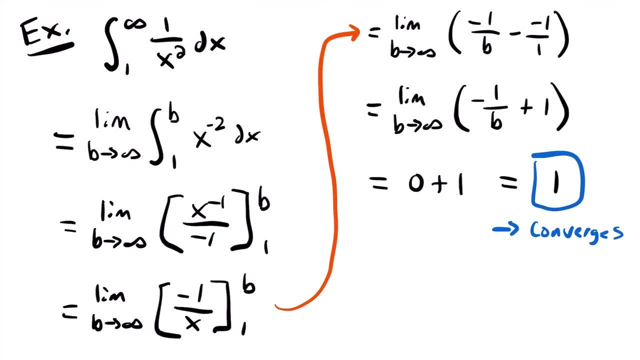 here for this integral. Remember that a definite integral calculates the area underneath that function, between the bounds of integration, And so in this case, if we were to graph one divided by x squared, I'll draw our coordinate system here. This is going to be the y axis. 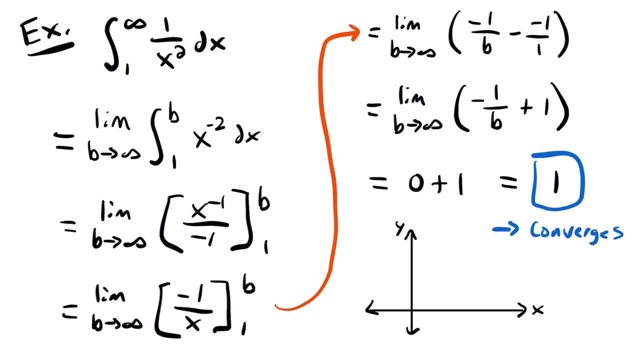 and then we will have the x axis. One divided by x squared has two parts. We have a curve on this side of the y axis and then another curve on this side of the y axis. So this is y equals one divided by x squared. We'll say that x equals one is right about here. 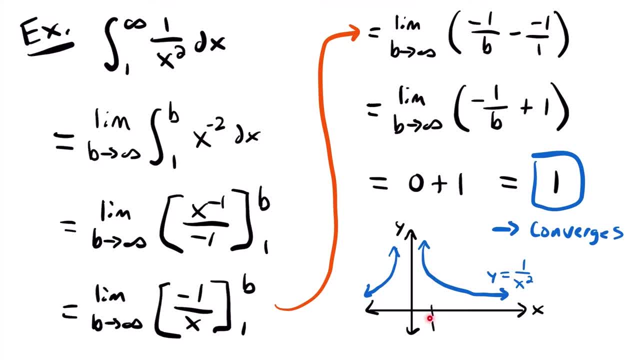 and we calculated the area beneath this function from that value of one to infinity, And so what I'm shading in represents the area that we just calculated that eventually converges to one. This area will continue on forever as this curve gets closer and closer to the x axis, And as you. 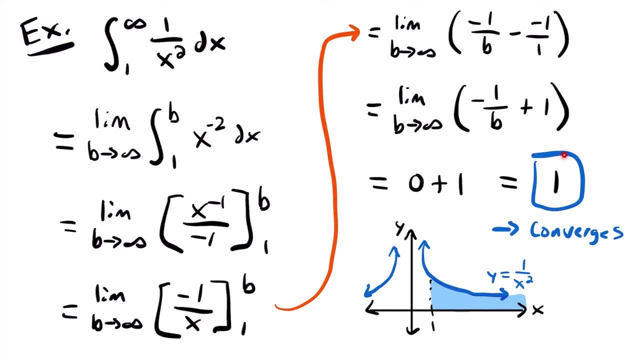 would add up all of that area. it would eventually add up to one as x approaches infinity. Okay, so hopefully this helps you visualize a little bit what's going on. here We're just calculating the area of an unbounded region, And sometimes that will converge to a specific value, such 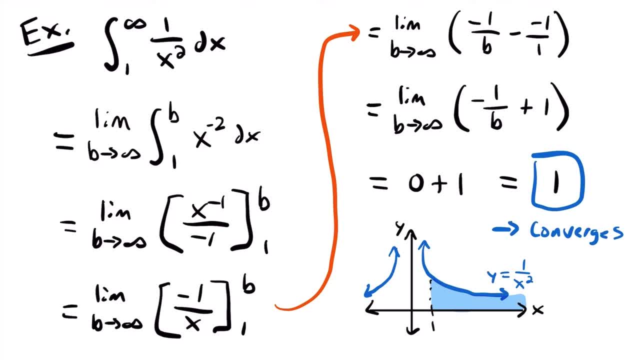 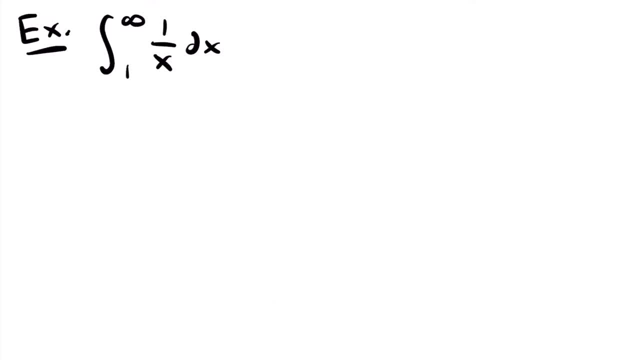 as one, But other times it's not going to converge to any value, and so it will diverge, And so let's take a look at an example of an integral where that is the case. Alright, so here's our second example. 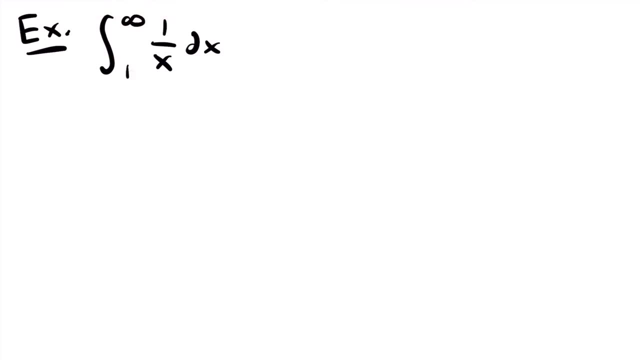 We have the integral, from one to infinity, of one divided by x- dx. Now, once again, this is an improper integral, because the upper bound is an infinite bound. We have infinity, and so we know that we need to introduce a limit in order to solve this integral. And 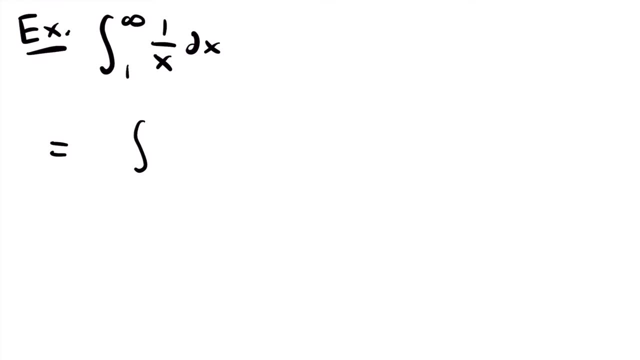 so let's set that up, Let's rewrite this. We're going to have the integral from 1 to b of 1 divided by x, dx, but then we need to take the limit as b approaches infinity. So we replaced infinity with b and then we introduced this limit of the integral as b. 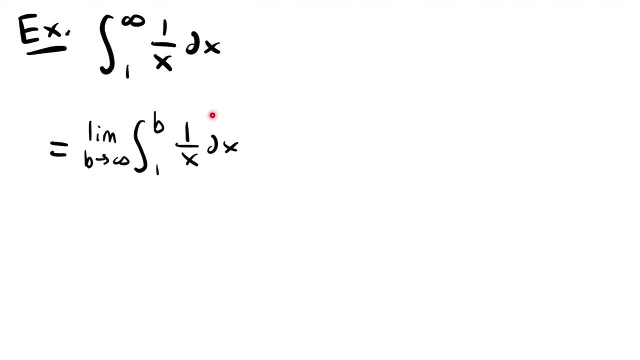 approaches infinity. Okay, so now let's integrate our integral here. We know from the log rule of integration that 1 divided by x is equal to the natural log of the absolute value of x, and so this is equal to the limit, as b approaches infinity, of the natural log of the absolute value of x, evaluated from 1 to. 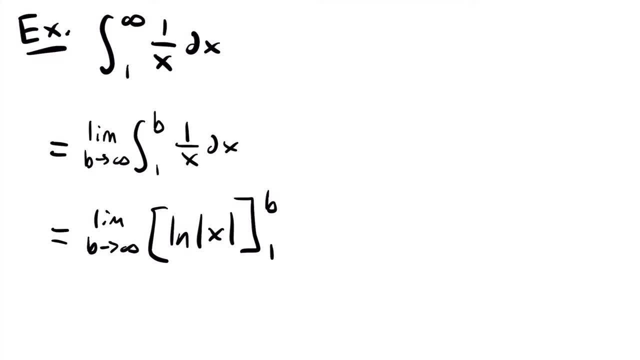 b. Now, in this case, we know we're working with all positive values, since we are integrating from 1 to infinity, or, in this case, 1 to b, but b can only be positive values, since we are starting at 1 and going towards positive infinity. 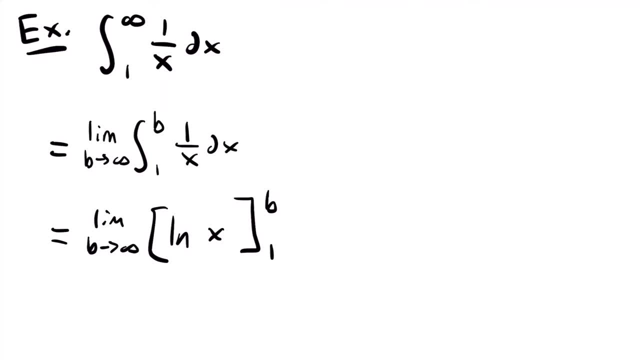 And so we actually don't need these absolute value bars. we can just have the natural log of x, because we don't need to worry about any negative values. But now, if we evaluate the natural log at b and subtract the evaluation at one, we will find that this is equal to the limit, as b approaches infinity of the. 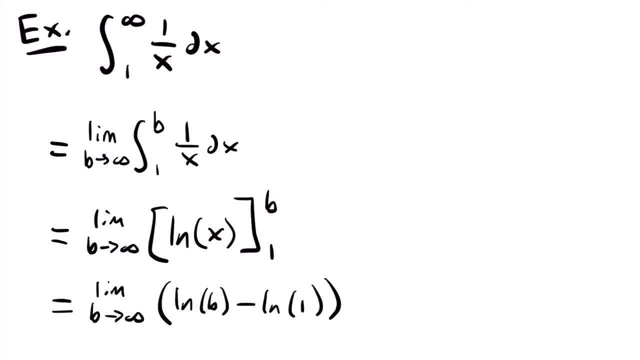 natural log of b minus the natural log of one, And so if we simplify that, this will be equal to the limit as b approaches infinity of the natural log of b, because the natural log of one is just equal to infinity, to 0.. When you plug 1 into the natural log function, the output is 0. And so we. 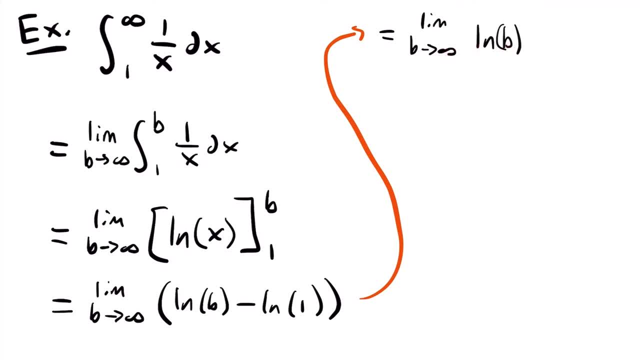 have the limit, as b approaches infinity, of the natural log of b. and so what happens to the natural log function as b approaches infinity? Well, as the value of b gets larger, the natural log function is going to output a larger value. For example, the natural log of 10 is approximately equal to 2.3025, and some 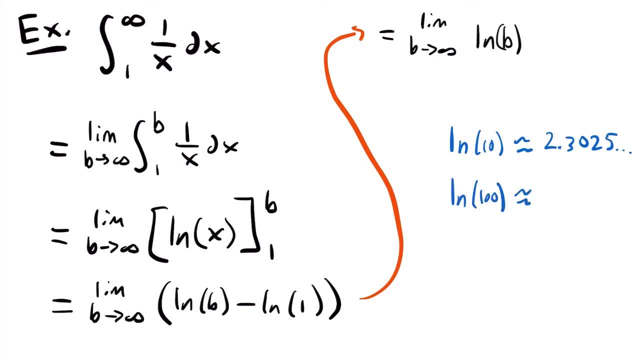 more decimals- The natural log of 100 is approximately equal to 4.605- and some more decimals, And as you would pick larger values to plug into the natural log function, it would continue to output a larger value. And so we can conclude that as b approaches infinity for the natural log function, the natural log. 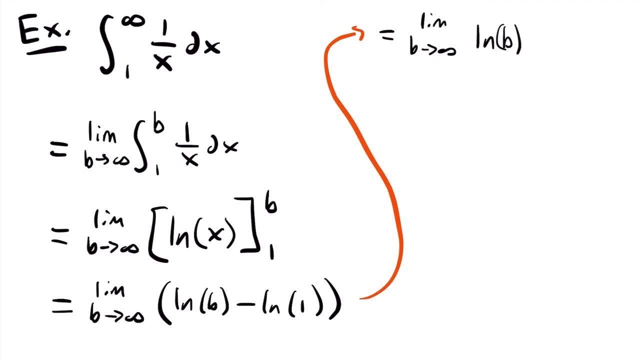 function itself will also become larger and larger towards infinity, and so we can say that this limit is equal to infinity. And so infinity is the solution to this improper integral, but it's not a finite value, and so we will say that this integral diverges, It does not settle. 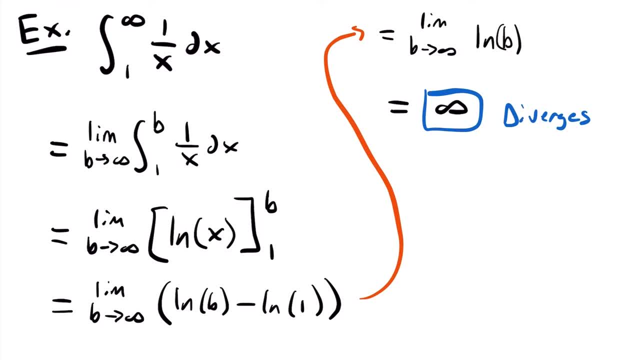 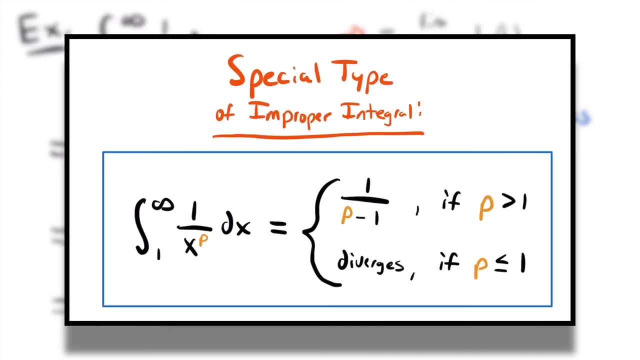 at a specific finite value, and so it does not converge, it diverges, And so we would say that this improper integral is divergent. Alright now, without even realizing it, the last two examples introduced you to a special type of improper integral that we sometimes call. 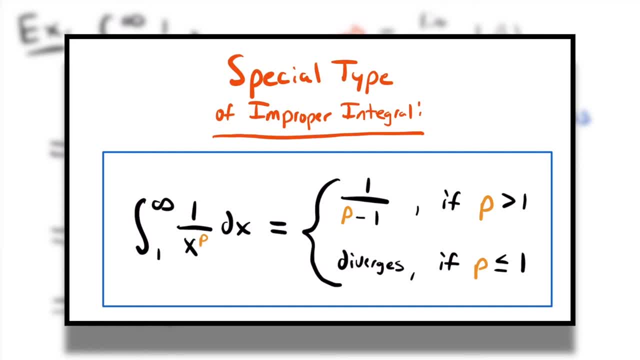 call a p-series Now. you'll learn more about what a p-series is later on in calculus, but for now this is all you need to know about this special type of improper integral. If you have the integral from 1 to infinity of 1 divided by x to some power, p times dx there. 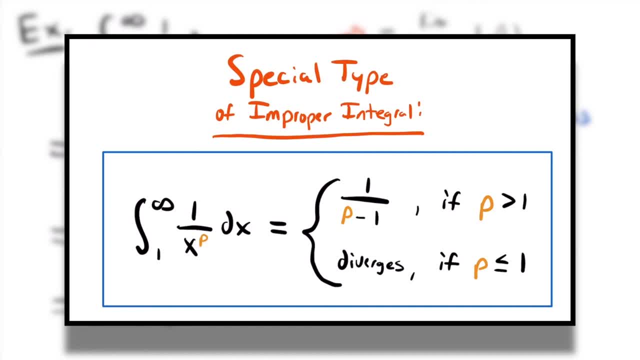 are two different possibilities for the solution to that improper integral. If the power, p right there- is greater than 1, then the improper integral will converge to a value of 1 divided by p minus 1.. However, if p is less than or equal to 1, meaning that power is less than. 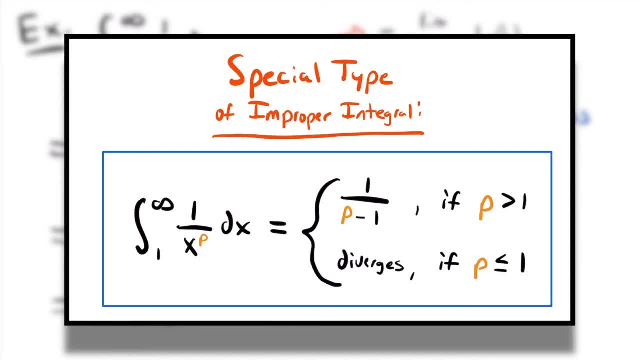 or equal to 1, then the improper integral will diverge and not converge to a specific value. Alright, and so you saw this. with our previous two examples, when we had 1 divided by x to the first power, we found that it diverged, which makes sense, because p was equal to 1. 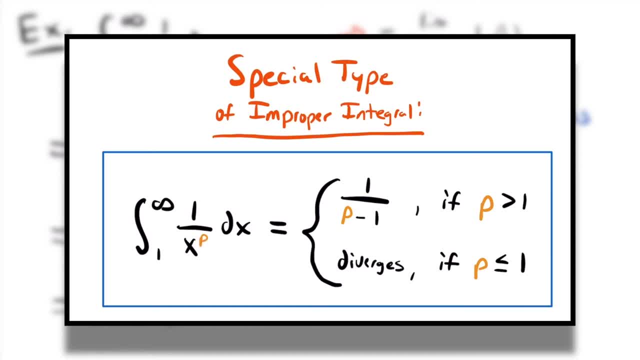 but when we had 1 divided by x, squared from 1 to infinity, then it converged to a value of 1.. And so our power was 2. so 2 minus 1 is equal to 1, and 1 divided by 1 is equal to 1.. Alright, 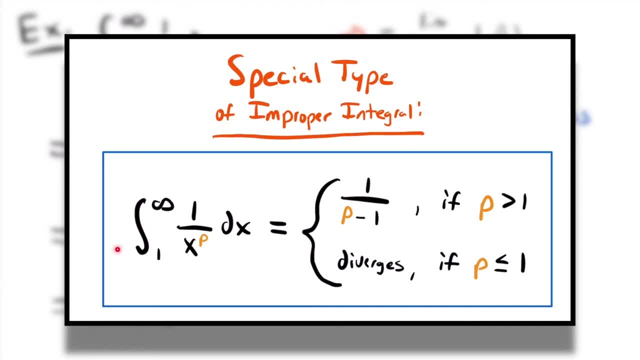 so maybe make a note of this. You might come across more examples of this type of an improper integral, and if you know what it can be equal to based on that power, it can certainly save you some time and you don't have to write out as much work. Alright, so this is a little. 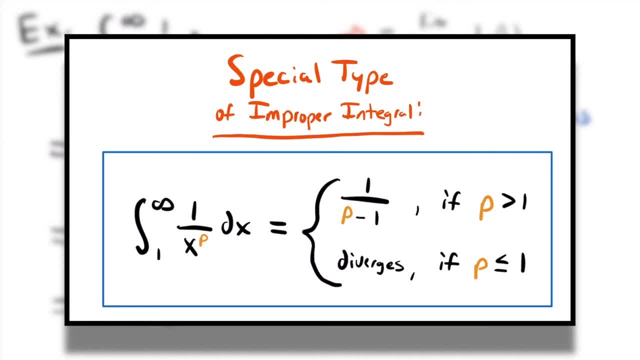 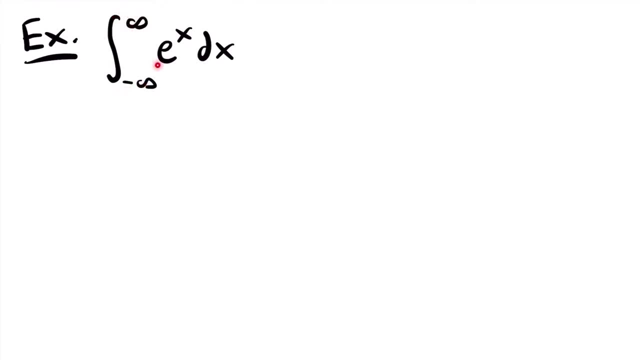 bit of a side note, Let's go back to more examples of solving improper integrals. Alright, so here's our next example. We have the integral from negative infinity to infinity, of e, to the power of x, dx. Now, in this case, it should be obvious that we have an improper. 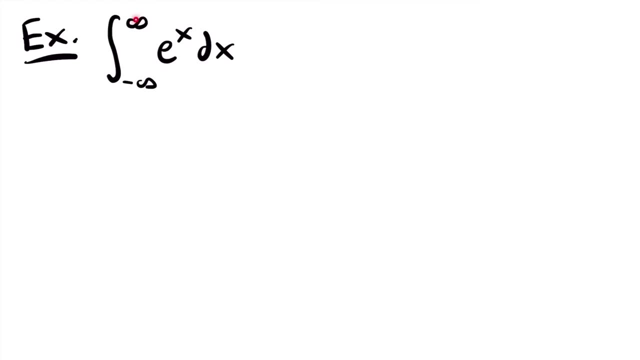 integral, because both of our bounds are infinite bounds, so that's a huge indicator that we have an improper integral, and so, unlike our previous examples, we actually have a step that we need to do before we can rewrite our bounds, with a limit, Since we are integrating. 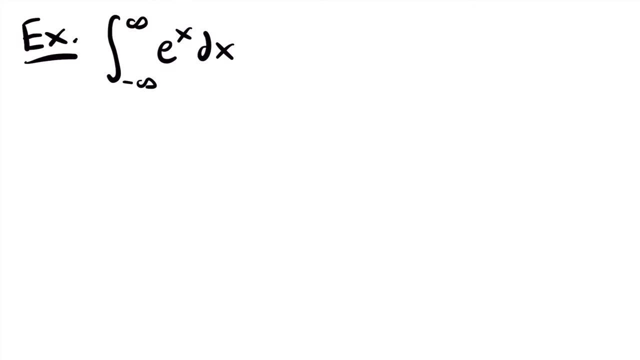 from negative infinity to infinity. we need to break up this integral into two separate integrals, So we have a value between negative infinity and infinity. Now e to the power of x is continuous for all values of x, and so really, you could choose any value of x you'd like to split. 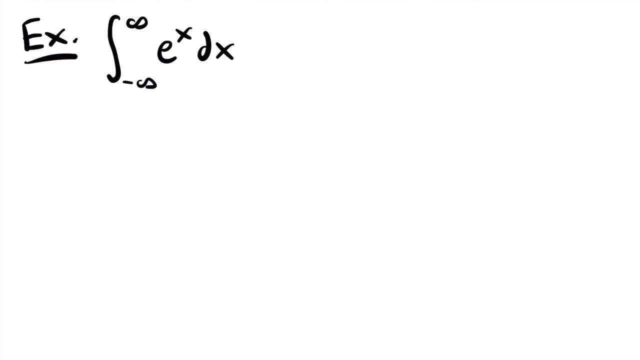 up this integral, but I'm just going to choose zero because that's a simple value to work with, and so what we'll do is rewrite this integral to be the integral from negative infinity to zero, of e to the power of x, dx, and add that to the integral from zero to. 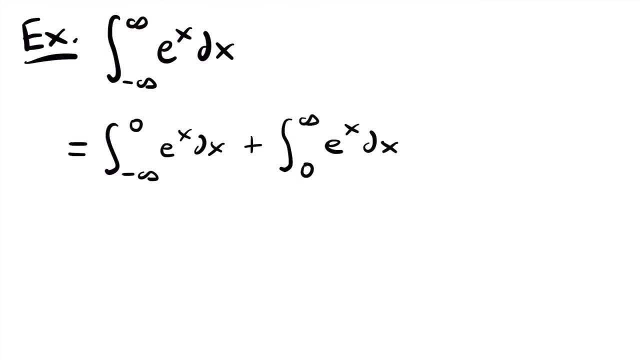 infinity of e to the power of x, dx, Right. So we chose a convenient value of zero. you could pick any other value if you wanted. you could pick one, you could pick two, you could pick negative a hundred, it doesn't matter. but zero is going to be a nice value to work with when we evaluate our integrals. Okay, 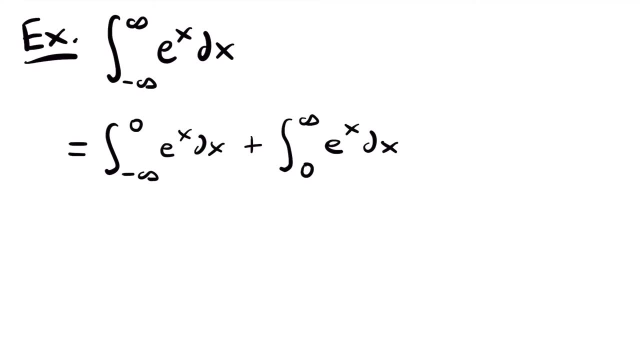 so you pick some value between negative infinity and infinity and then you split up the integral into two integrals where you integrate from negative infinity to that convenient value and then add that second integral where you integrate from that value to positive infinity. All right, So we can rewrite both of these integrals by replacing our infinite bounds with a and. 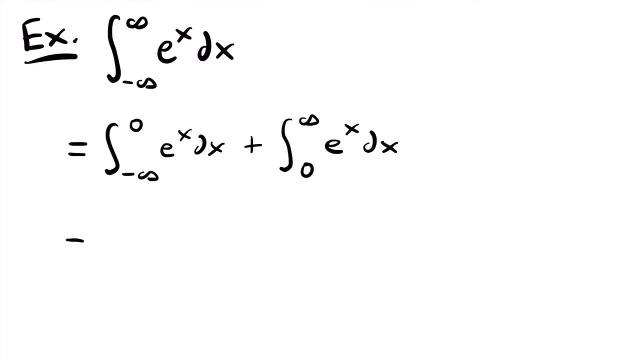 b and then introducing a limit. So we'll have that this is equal to the integral from a to zero of e to the power of x, dx. but then we need to take the limit of that integral as a approaches negative infinity and we will add that to the integral from zero to b of 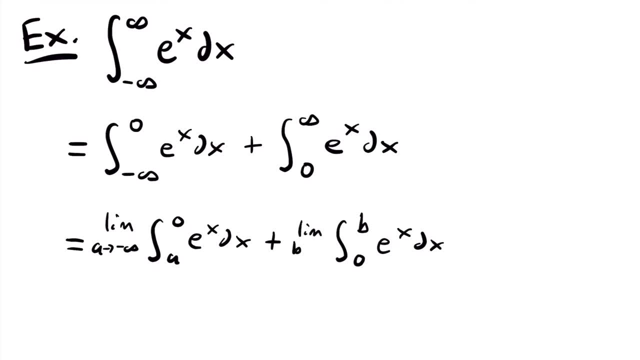 e to the power of x dx, where we will now have the limit as b approaches positive infinity. Okay, So we replaced negative infinity with a, and now we have the limit as a approaches negative infinity. and we replaced infinity with b, and now we have the limit as b approaches infinity. 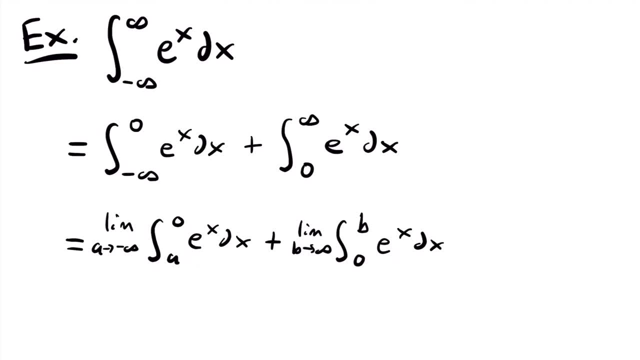 for that integral. All right, so now, if we evaluate both of our integrals here, the integral of e to the power of x is just itself, and so we'll have that this is equal to the limit as a approaches negative infinity of e to the power of x, evaluated from a to zero, plus the limit as b approaches. 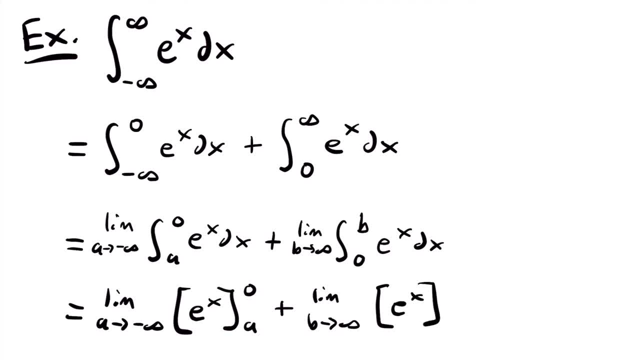 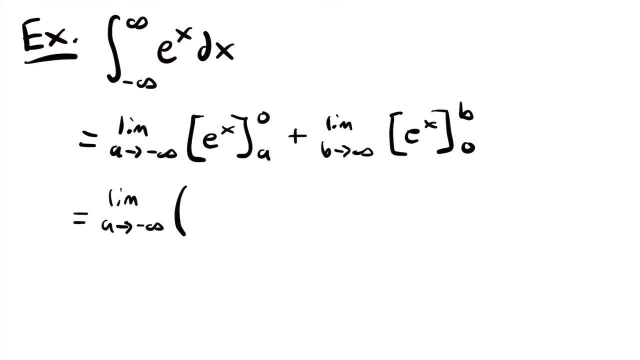 positive infinity of e to the power of x, evaluated from zero to b. Now, if I clean up my work here, we can now evaluate e to the power of x in both cases at their bounds. so if we do that, this will be equal to the limit as a approaches. negative infinity of e to 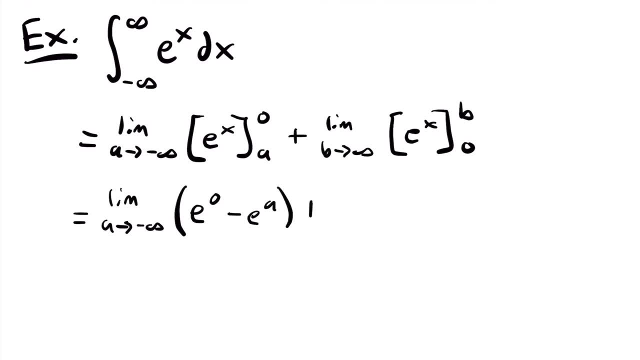 the power of zero minus e to the power of a plus the limit as b approaches positive infinity. of e to the power of b minus e to the power of zero. Okay, So e to the power of zero in both instances is just equal to one, because any constant. 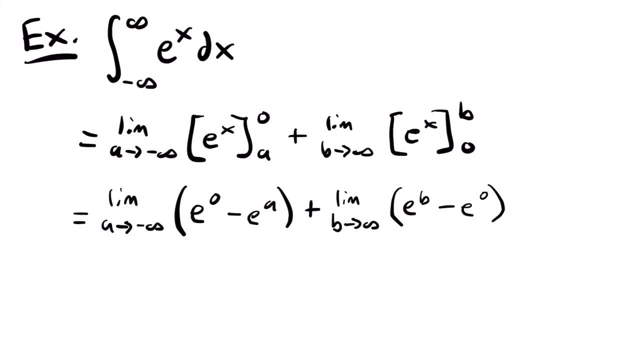 raised to the power of zero is equal to one other than zero, of course, and so I'm just going to rewrite both of those to just be one. so we will have one minus e to the power of a and e to the power of b minus one. 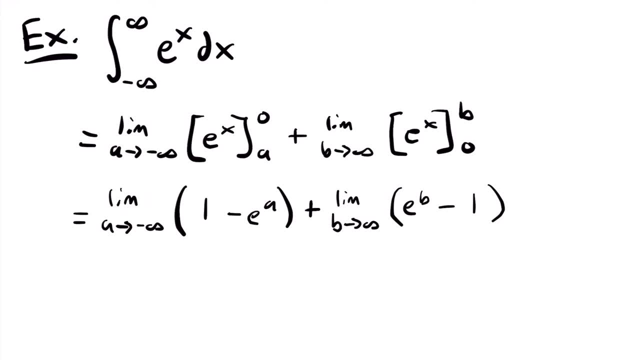 All right, and now we can look at each of these limits individually. We have the limit, as a approaches negative infinity, of one minus e to the power of a. so if a approaches negative infinity, Then we have e to the power of a. what is going to happen to this value as that power becomes? 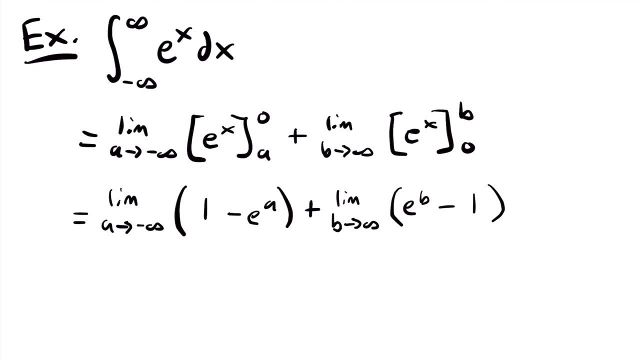 a greater and greater negative value. Well, as you raise e to a higher and higher negative value, e is going to become closer and closer to zero. if you have e to the power of negative one, that is approximately equal to zero point three, six, seven, eight, seven and some more decimals and e to the power, 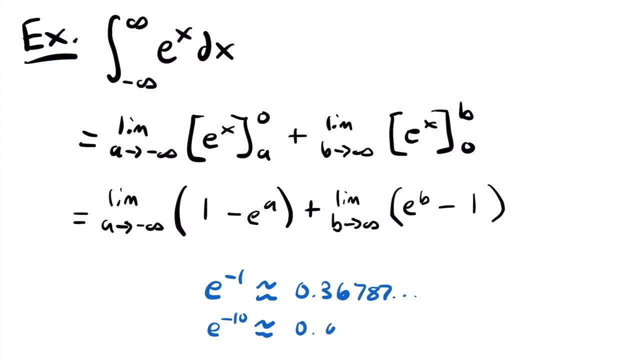 of negative ten is approximately equal to zero point zero point eight, and so on, Okay, Okay. So we have e to the power of zero, zero, zero, zero, four, five, four and some more decimals, and so, as you pick a larger negative value to be the exponent of e, it is getting closer. 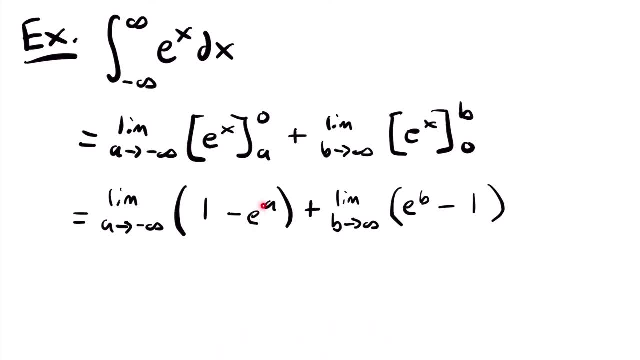 to zero, and so we would say that e to the power of negative infinity, if you will, is equal to zero, and so we will have that this is equal to one minus zero for that first limit, right? just remember that the limit as a or x approaches anything of a constant is: 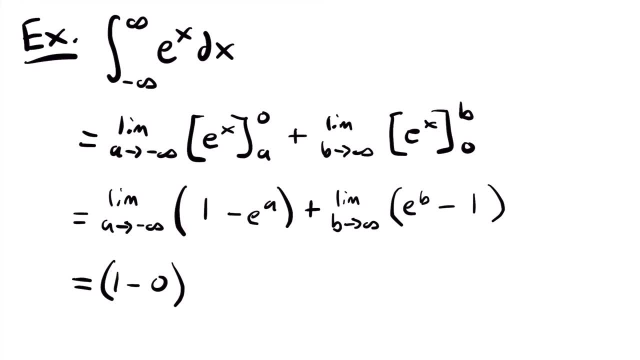 just equal to that constant. So that's why we just have one minus zero. now for a second limit. here we have the limit as b approaches infinity of e to the power of b minus one, and as the power of e reaches towards positive infinity, as this power gets greater and greater that whole term will get. 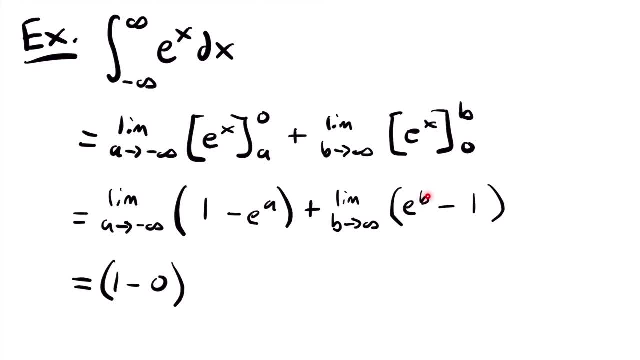 larger towards infinity, and so we would say that e to the power of infinity is just going to be infinity. so we have plus infinity, and then the limit of negative one is just the negative one, and so we have one plus zero, plus infinity, minus one that will be equal. 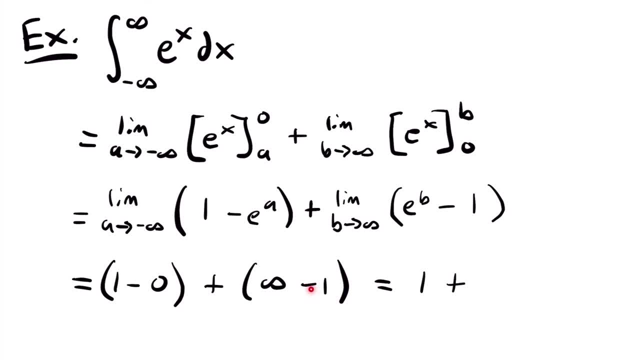 to one plus infinity. minus one is still infinity, and so we have one plus infinity, but that's still equal to infinity as well, and so, even though one of those limits converge to one and this limit would have diverged to infinity, when we add them together we still have a. 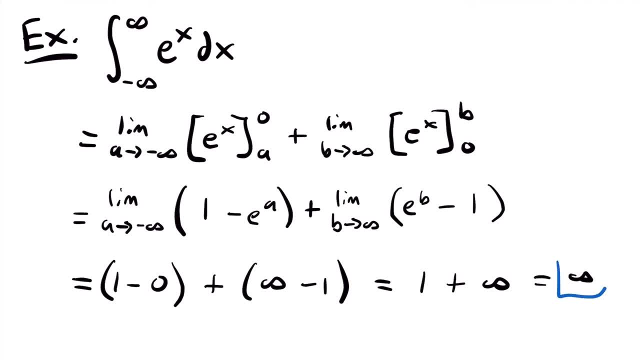 divergent solution. our improper integral is equal to positive infinity, but the improper integral still diverges. okay, so even though we had two integrals and one of them converged and the other one diverged, the original integral itself is going to diverge in order for it. 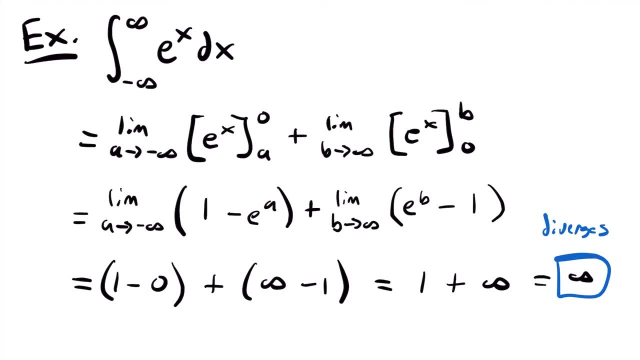 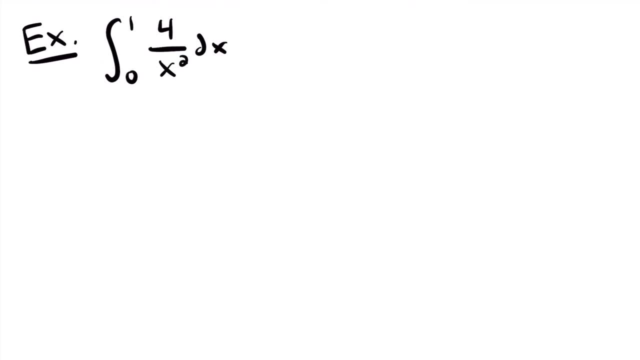 to be convergent. both of those resulting integrals that we split it up into need to be convergent themselves. Let's take a look at another example. alright, so next up we have the integral from zero to one of four, divided by x, squared dx. now, initially this may just seem to be a regular 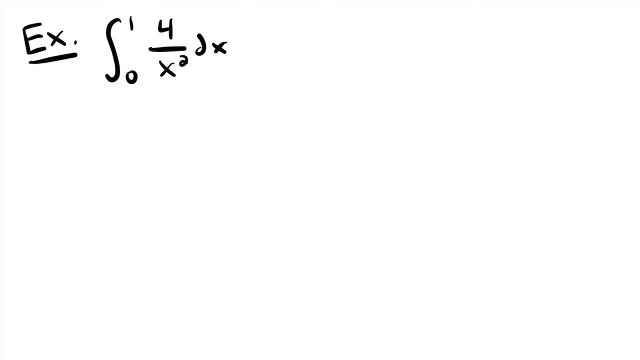 definite integral. This is the integral that we have been evaluating all through calculus. however, this is actually an improper integral. it is the second type of improper integral, where we have an infinite discontinuity, or in other words, our function is going to be undefined for some value between 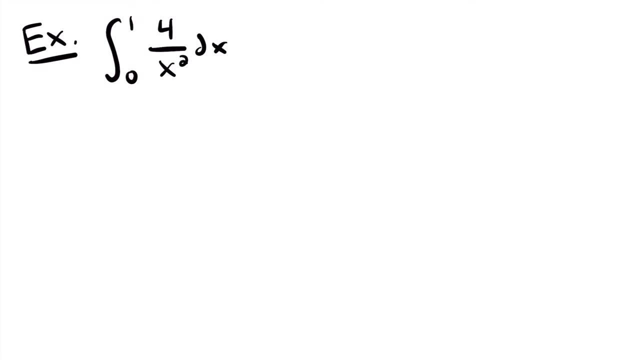 our bounds, and including the bounds. and so do you see where that discontinuity would be? Well, it's actually at the lower bound of zero. if you plug zero into this function, four divided by zero squared will be four divided by zero, and you can't divide by zero. so that would 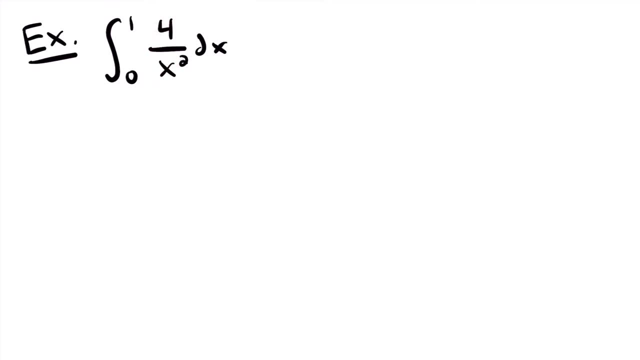 be an undefined value, and so four divided by x squared is undefined. at x equals zero. This function is not continuous for the range of values that we want to integrate it for, and you would see that if you looked at the graph of the function, it would look something. 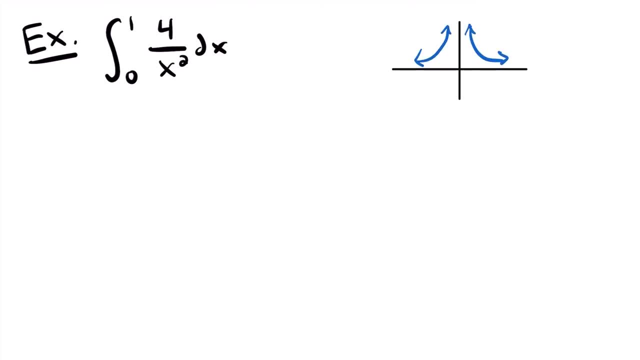 like this. I believe we looked at a function similar to this earlier, where it is not defined at x equals zero, Right, this function has a vertical asymptote. In fact, you can see from this graph here that the limit from either side of x equals zero. 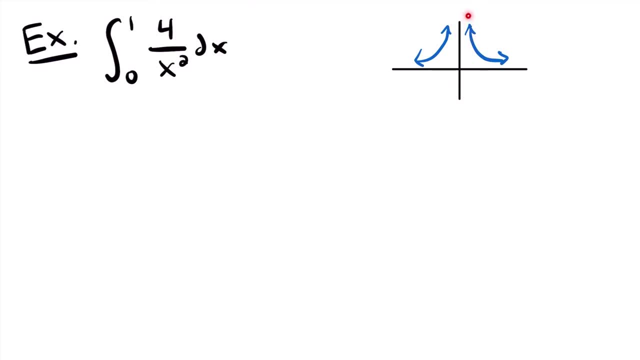 for that function would be positive infinity. Our function would increase towards positive infinity as it approaches. x equals zero, and so because of that, we cannot use our traditional method of solving this definite integral. we need to treat it as an improper integral, because that's what it is. 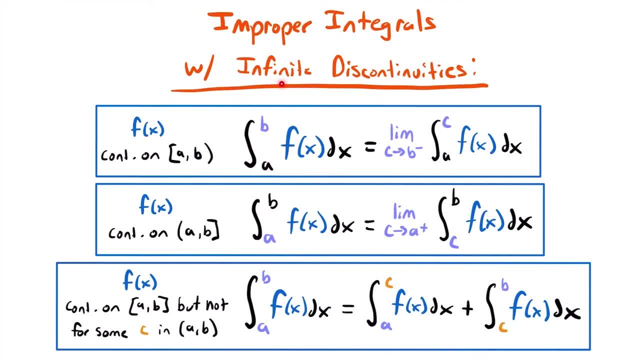 And so here's how we're going to deal with improper integrals that have infinite discontinuity, or when a function is not continuous for the range of values that we want to integrate it for. And so if our function is continuous from a to b, but b is not included, meaning it's 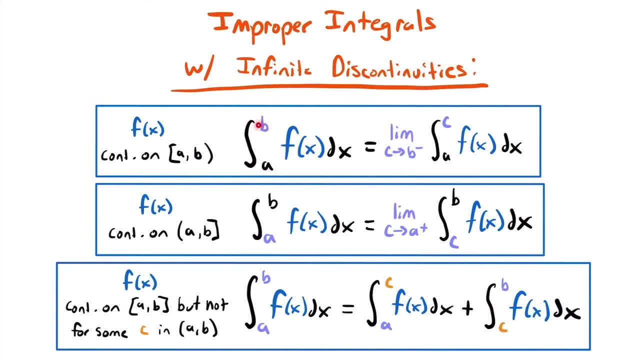 not defined at b, then you want to replace that bound b that the function is not defined at, with another value, c, and then take the limit as c approaches b from the left. Alright, so when you replace the upper bound, you're going to have the limit of that value. 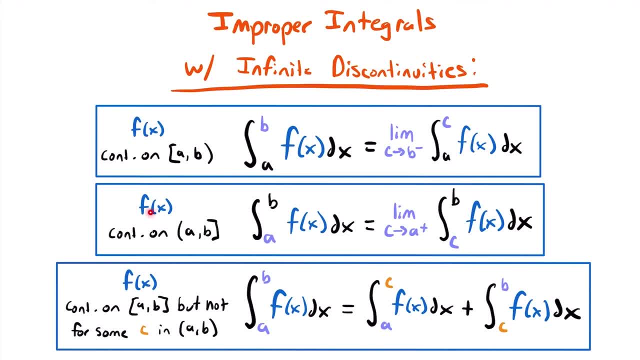 from the left side of the function. You have an integral where the function is continuous from a to b but not including a, meaning it is undefined at that value of a. then you want to replace a with another value and then take the limit of that value as it approaches a from the right side of that value. 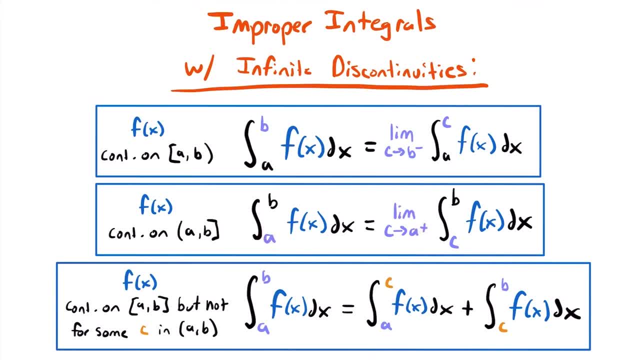 Okay. so if you're replacing the lower bound, you take the limit as you approach the right side of that value. And then let's say you have an integral where the function is continuous on the interval but not at a specific value of c. So you want to replace that value of c between those two values, a and b. 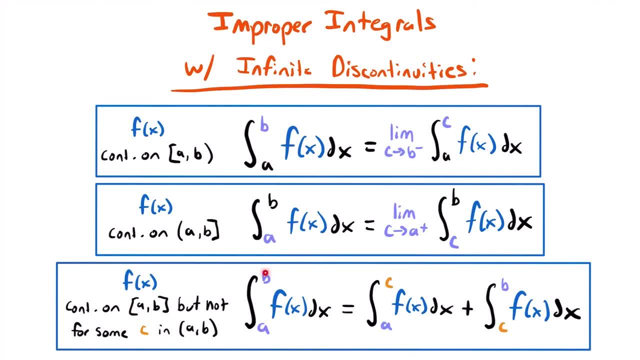 Right, so this function maybe is continuous for both of those bounds of integration, but it's not continuous at a point between them. then you would need to split it up into two integrals where that value of c is where the function is not continuous, And so then you would rewrite each of these integrals using the previous two rules. 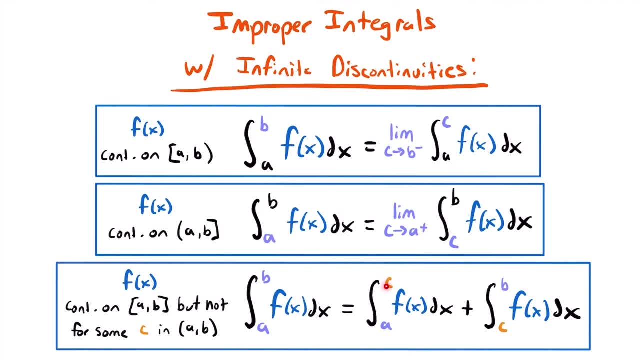 You would replace those bounds where the function is not continuous with another value and then take the limit of that new value as it approaches c. Okay, so that's the first thing we're going to do. We're going to take the value of c from either the left or the right. 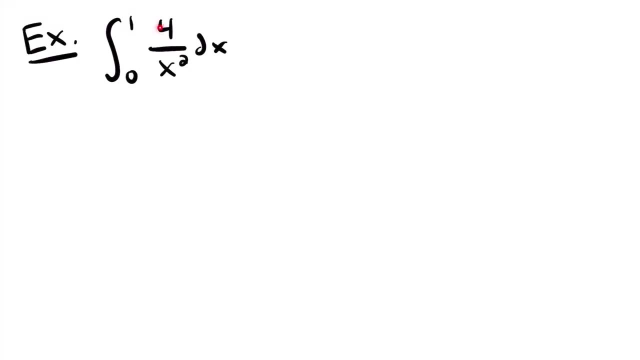 Okay, and so let's go back to our example. Remember we said that four divided by x squared is not defined, for x equals zero. So we're going to replace zero with another value and then have the limit of that value as it approaches zero from the right side. 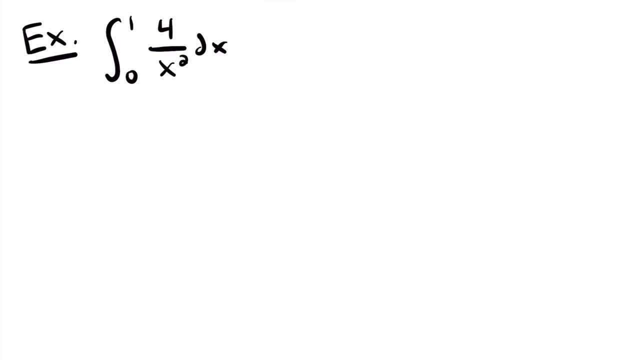 Okay. so remember, when you replace the lower bound, you take the limit as you approach that value from the right, But if you replace the upper bound, you take the limit as you approach that value from the left, And so this will be equal To the integral from a to one of four divided by x squared dx, and then we will take the. 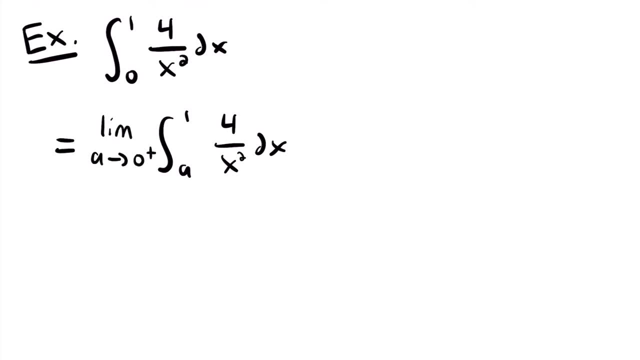 limit as a approaches zero from the right, And so now let's work on solving this integral. We have four divided by x squared. If we move x squared to the numerator and make the exponent negative, we will be able to see how we can integrate this using the power rule. 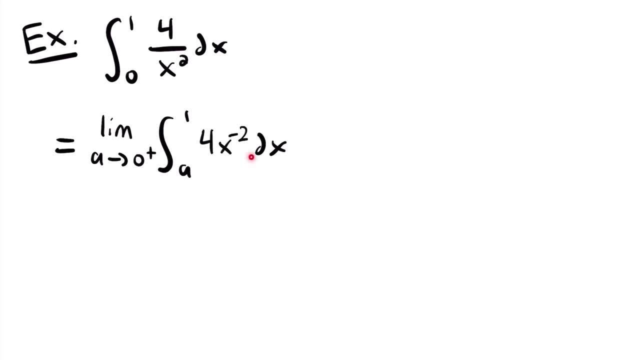 So we have four times x to the negative second power, And so then we can integrate by adding one to that exponent and dividing by that new exponent. So this will be equal to the limit as a approaches zero from the right of four times x to the. 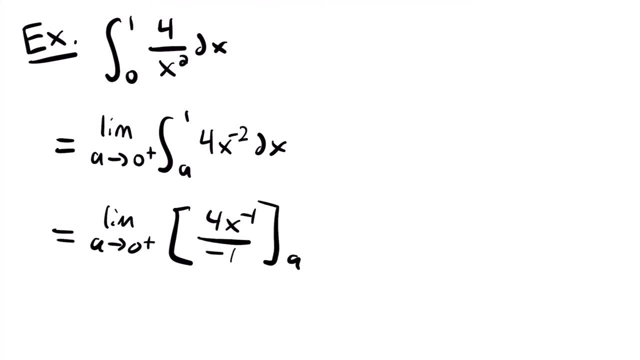 negative. first power divided by negative one, evaluated from a to one. Okay, so negative two plus one is negative one, and then we divide by that new exponent of negative one. Now, if we rewrite this a little bit, four divided by negative one is negative four, and then 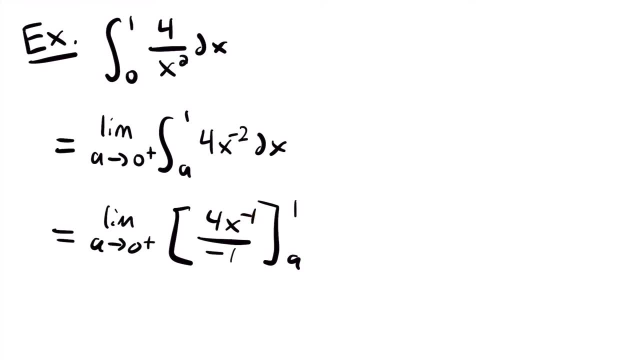 we can move x to the negative first power, to the denominator, and make it x to the positive first power. So this will be equal to the limit as a approaches zero from the right of negative four divided by x, evaluated from a to one. Now, if we continue our work up here, we can now evaluate this expression at one and subtract. 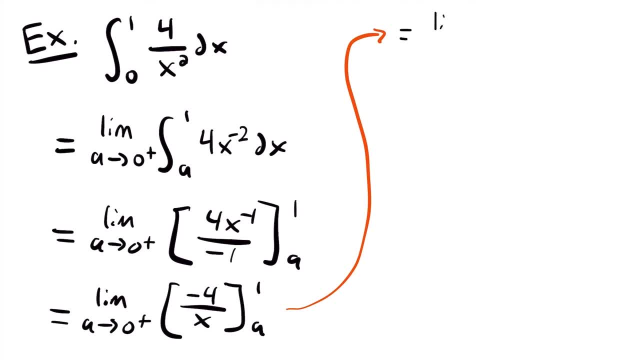 the evaluation at a, And so this will be equal to the limit, as a approaches zero, from the right, of negative four divided by one, minus negative four divided by a Right. so we plugged one in for x, So we have negative four divided by one. 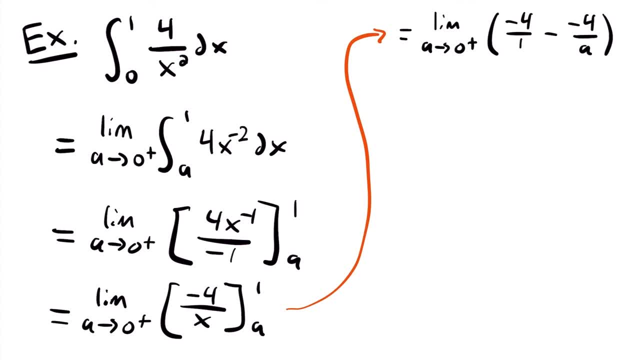 And then we plug in a for x, and so we have negative four divided by a. Now negative four divided by one is just negative four. So I'll rewrite that We'll have negative four and then these two negatives will cancel out to become positive. 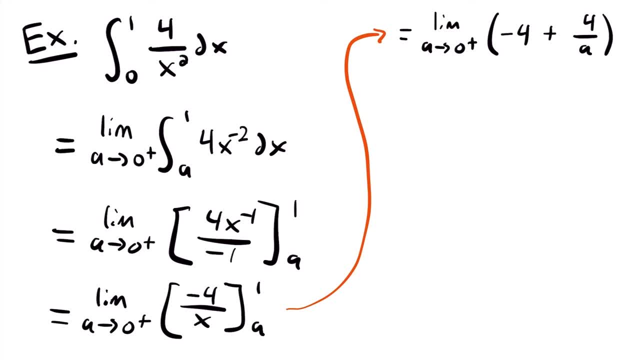 and so we'll just have plus four divided by a, And now we can take the limit of both of these parts, and any limit of a constant is just going to be equal to that constant. So this will be equal to negative four plus the limit as a approaches zero from the right. 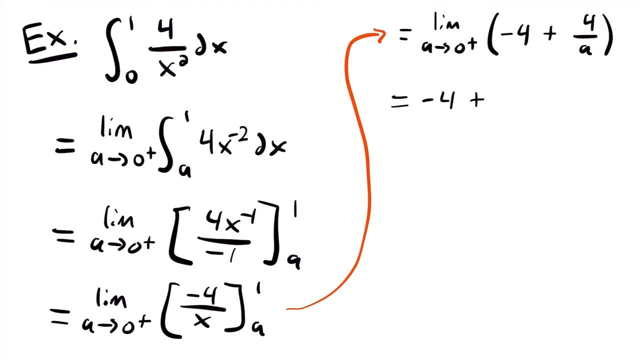 of negative four divided by a. Now, when you have a one sided limit, the first thing that you should try to do is plug in that value, but four divided by zero is undefined, So that's not going to work. What we have to do instead is see what happens to this expression as we pick values of a. 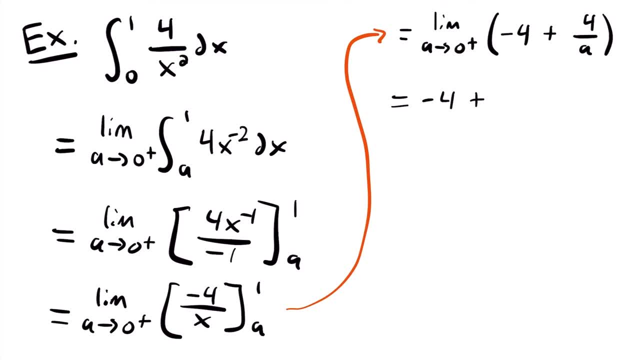 that are closer and closer to zero from the right side. So that means we're going to be picking positive values that get closer to zero. And so let's say: a is equal to zero point one. That would give us four divided by zero point one. 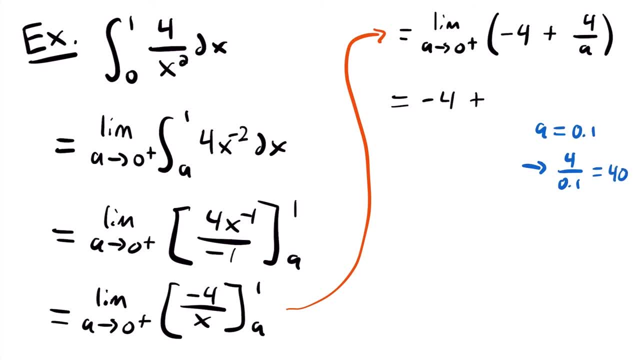 And then we'll have negative four divided by a, Which is equal to forty. If we let a be equal to zero point zero, one which is even closer to zero from the right, then we will have four divided by zero point zero, one which is equal to four hundred. 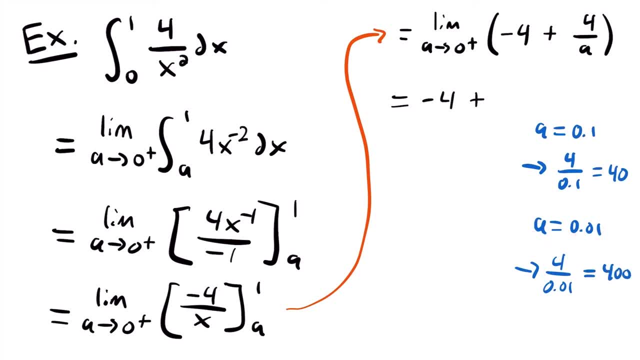 Now, if we let a be equal to zero, point zero, zero one, then we would have four thousand and so on. So as we pick values of a closer and closer to zero from the right side, this fraction gets larger towards infinity, and so we would say that the limit as a approaches zero from. 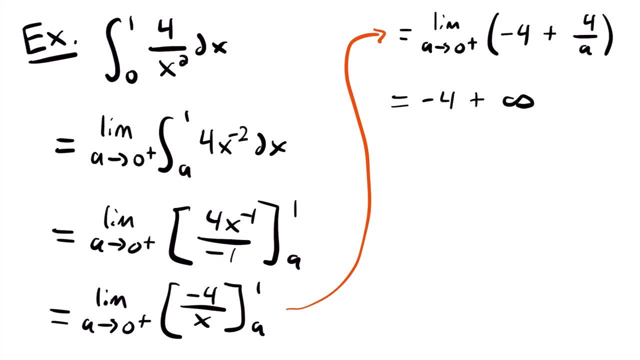 the right of four divided by a is infinity, And so negative four plus infinity is still infinity, and so we find that the solution to our improper integral is positive infinity. And so, while that is the solution, our improper integral in this case diverges. It does not converge to a specific finite value. instead, it's an infinite value, and so 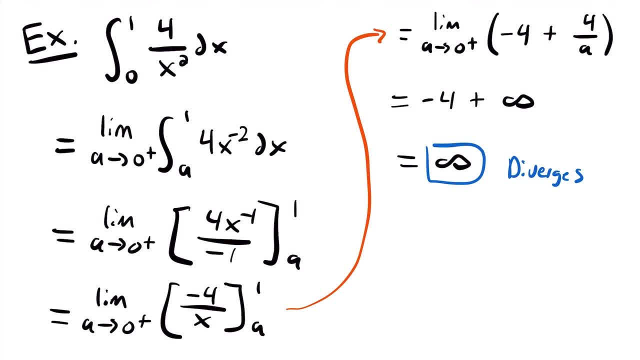 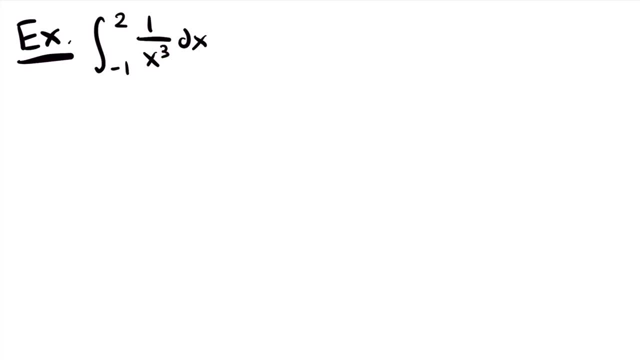 it diverges. Okay, Let's look at one more example for this video. Alright, so here's the last example. We have the integral from negative one to two of one divided by x, cubed times dx. Now, similar to our previous example, this initially looks like a pretty nice integral that we 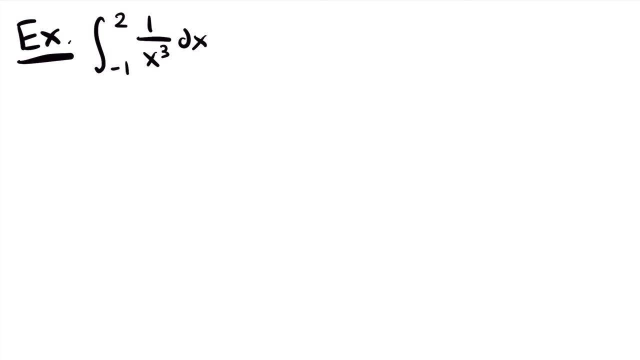 know how to solve. It doesn't look like anything special. However, one divided by x cubed is not going to be continuous for the entire range of values that we want to integrate it for. Now it is defined at negative one. Right negative one cubed is negative one. 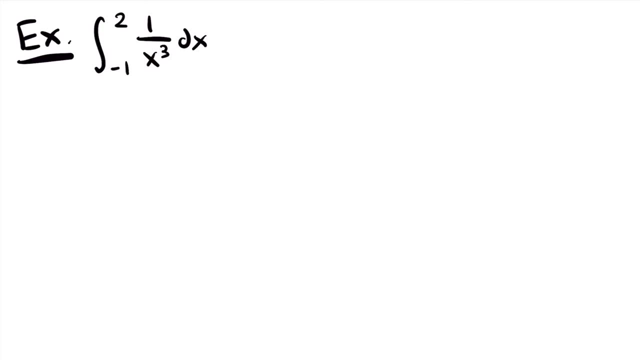 So one divided by negative one is just negative one. That's good. And if you plug two in, you have two cubed, and so you have one divided by eight, and so that's also good. But if we look at the values between negative one and two, is there a value of x for which 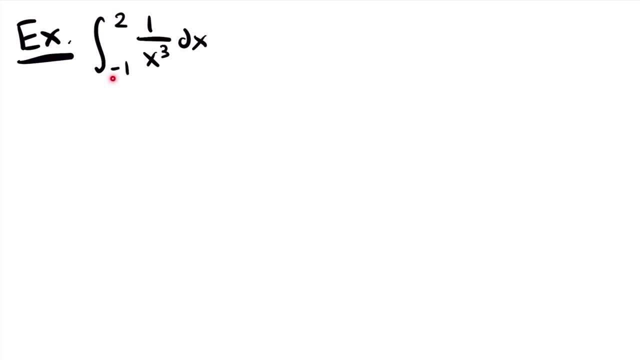 the function is undefined. Well, zero lies between negative one and two, and if you plug zero into this function- one divided by x cubed- you would have one divided by zero cubed, which is one divided by zero, and that's undefined. So this function- one divided by x cubed- is not defined at zero. 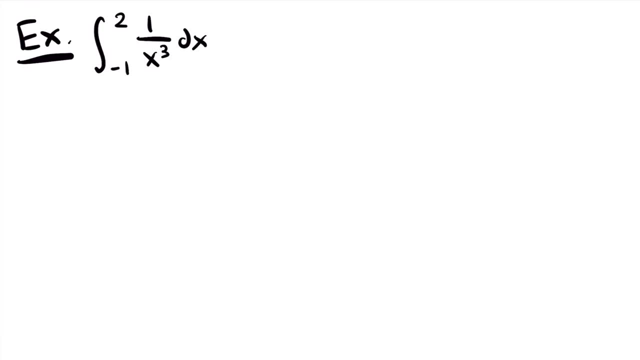 We have an infinite discontinuity at that point, And so we cannot evaluate this integral as normal. If you were to just integrate one divided by x, cubed, and then evaluate out your bounds of integration, you would get some other value. I think it's three eighths or something, and that would be incorrect. 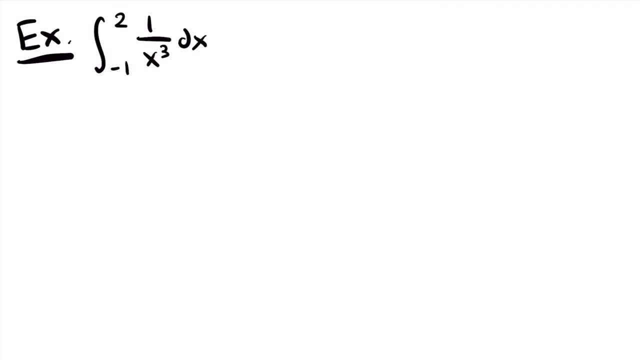 That is not the solution to this integral, because x cubed is not continuous for the range of values that we want to integrate it for, And so what we have to do is split up this integral into two separate integrals using that value that it is undefined at. 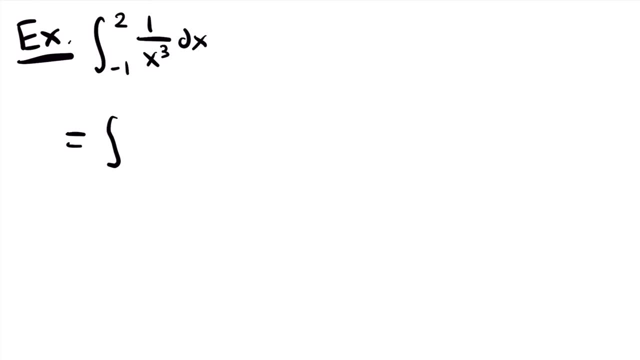 And so here's what we're going to have. This is going to be equal to the integral from that lower bound of negative one, to the value of x, where our function is undefined. So that's zero, and then we'll have one divided by x, cubed dx, and we're going to add that. 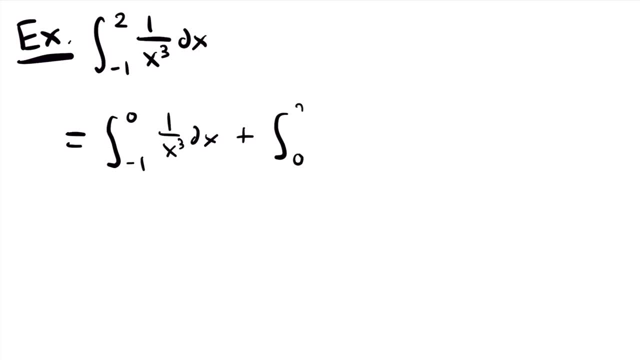 to the integral, from that value of zero to our upper bound of two, And so we'll have one divided by x, cubed times dx. And now what we need to do is rewrite each of these integrals by introducing a limit for that bound of integration that our function is not defined for. 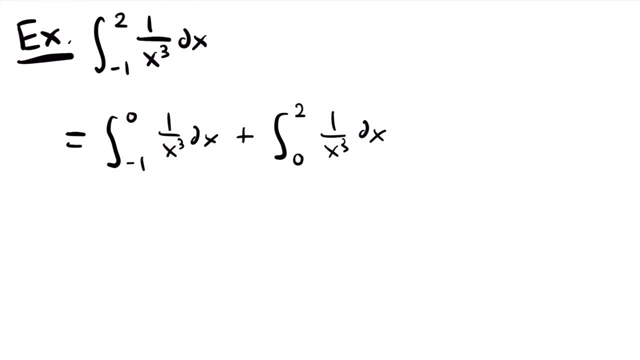 So we're going to replace each of these zeros with a different value and then take the limit of that value as we approach zero And, depending on whether it's the upper bound or lower bound, we're going to be looking at different sides of that function. 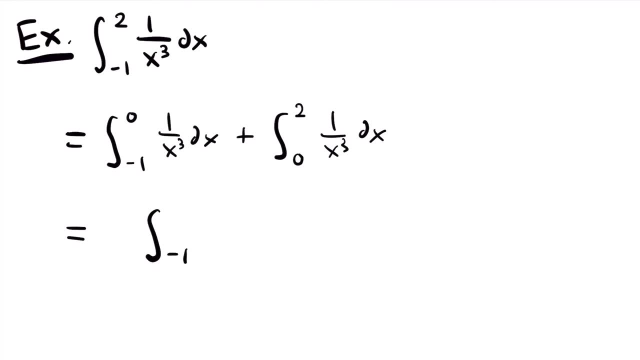 And so here's what that looks like. This will be equal to the integral from negative one to b of one divided by x cubed dx, And so we're going to have one divided by x cubed dx, And then we're going to take the limit as b approaches zero from the left. 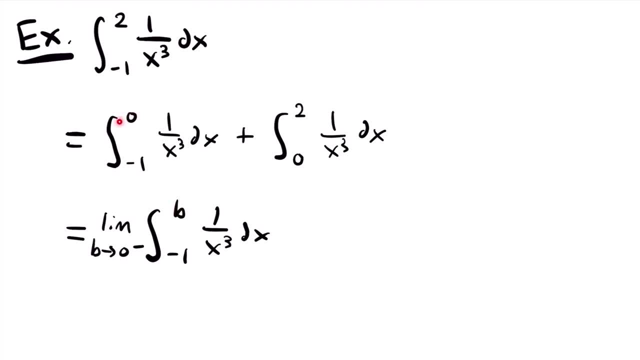 Okay, so we replaced zero with b and since that is an upper bound, we're going to take the limit as b approaches that value from the left side. Now for our second integral. we will add the integral from a to two of one divided by x cubed dx, and then we will have the limit as a approaches zero from the right. 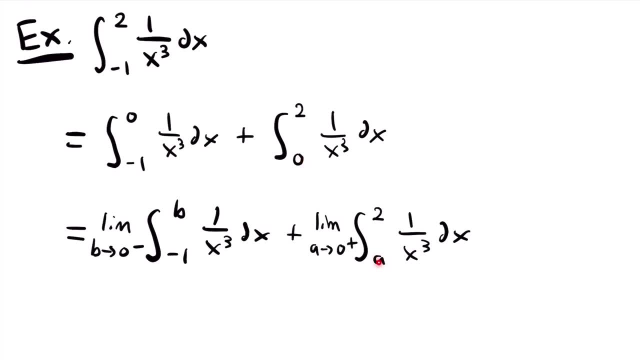 Okay, So we replaced zero with a, And since that is a lower bound, we take the limit as a approaches that value from the right. Okay, and so now we can work on integrating these two integrals. Note that in each case we have the same function, and so if we move x cubed to the numerator, 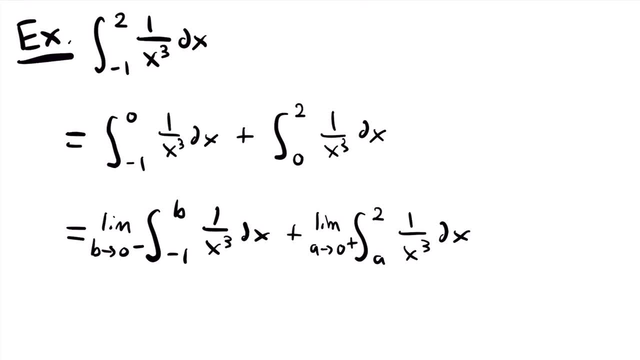 by making the exponent negative. we can then use the power rule of integration to integrate it. So I'm going to rewrite both of those. Instead of having one divided by x cubed, you will have x to the negative third power. And so now, if we integrate, 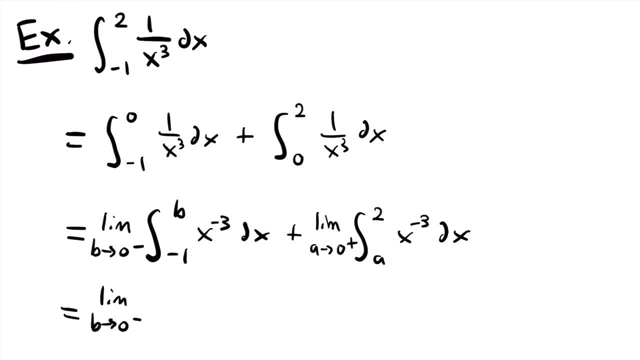 This will be equal to the limit as b approaches zero, from the left of x to the negative second power, divided by negative two, evaluated from negative one to b Right. we added one to the exponent, so we have negative two and we divided by that new exponent. 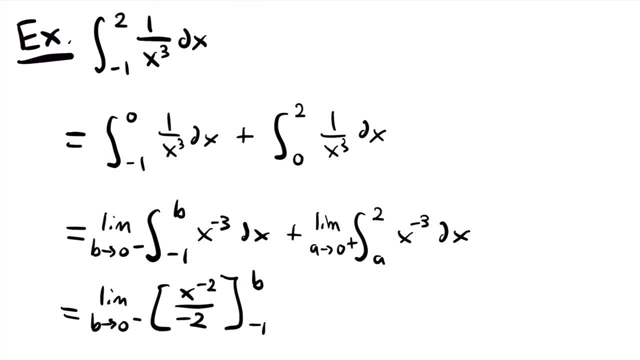 of negative two. Now we'll do the same thing over here. It's the same integral, but we do have different bounds of integration and a different limit. So we have plus the limit as a approaches zero from the right of x to the negative second. 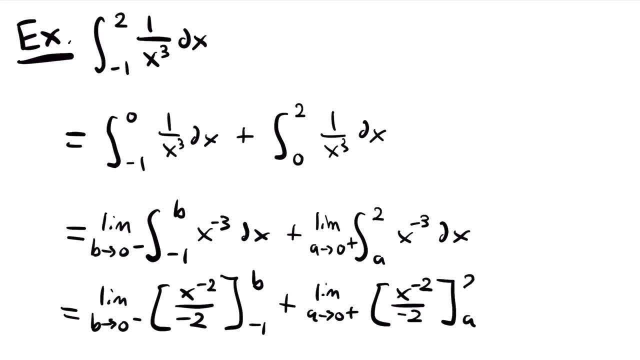 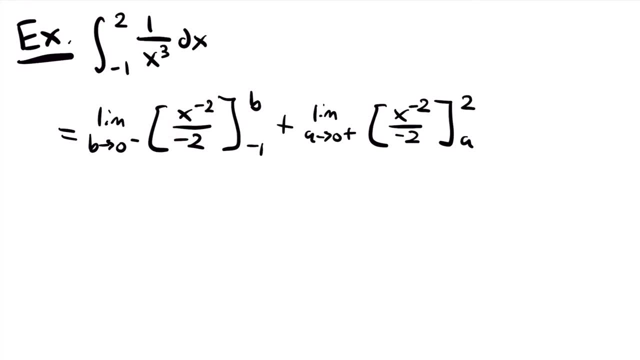 power, And so we'll have x to the negative, two evaluated from a to two. Okay, so now, if I clean up my work here, we can simplify this expression a little bit. We can move that negative to the numerator and then move x to the negative second power. 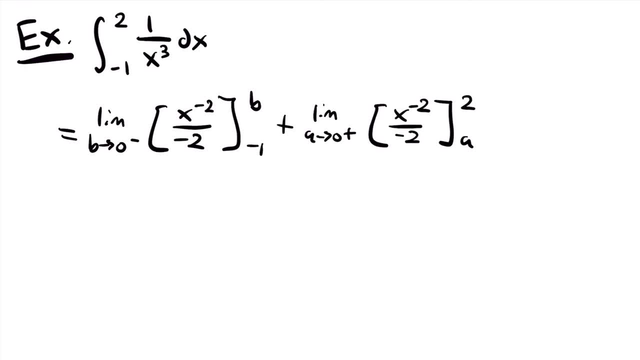 to the denominator by making the negative exponent positive, And so if we do that, this will be equal to the limit as b approaches zero from the left of negative one divided by two times x, squared evaluated from negative one to b. Now we'll do the same thing for this expression. 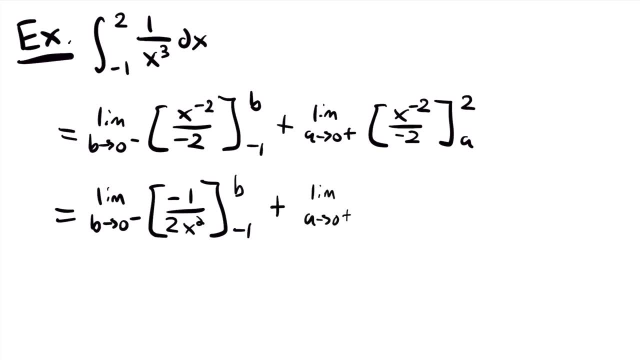 And so we'll have, plus the limit as a approaches zero from the right of negative one divided by two times x, squared evaluated from a to two. Okay, and so now we can evaluate each expression at its bounds of integration. We start by plugging in that upper bound and then subtract, plugging in that lower bound. 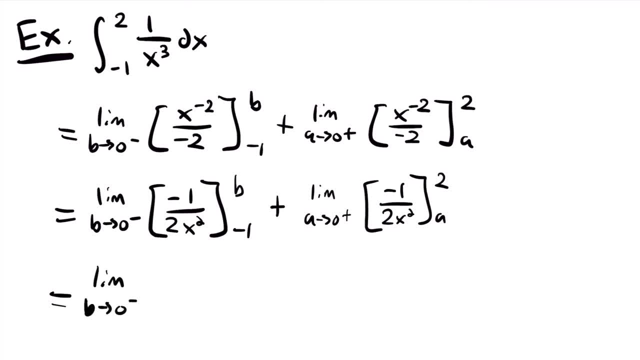 And so this is equal to the limit as b approaches zero from the left of negative one divided by two times b squared minus negative one divided by two times negative one. And then we will add our second limit as a approaches zero from the right of negative. 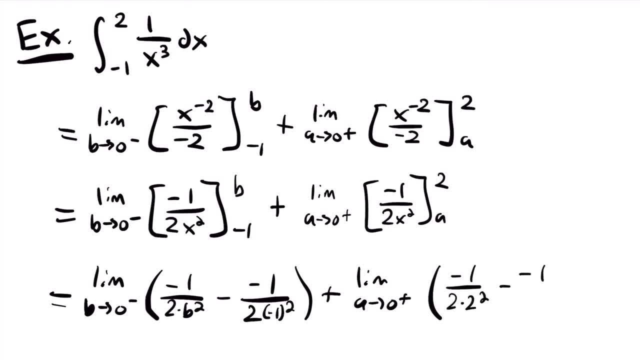 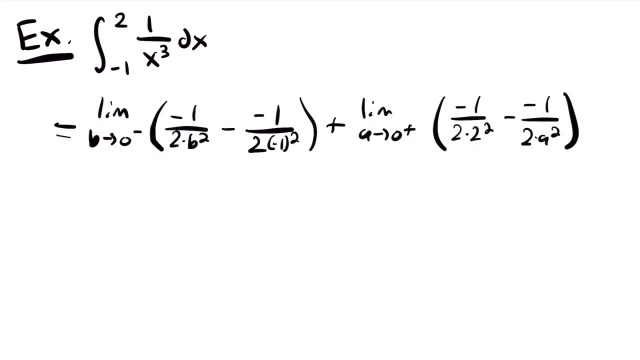 one divided by two times two squared, minus negative one divided by two times a squared. Now, if I clean up my work again, we can simplify a little bit. We'll have that this is equal to the limit as b approaches zero from the left of negative. 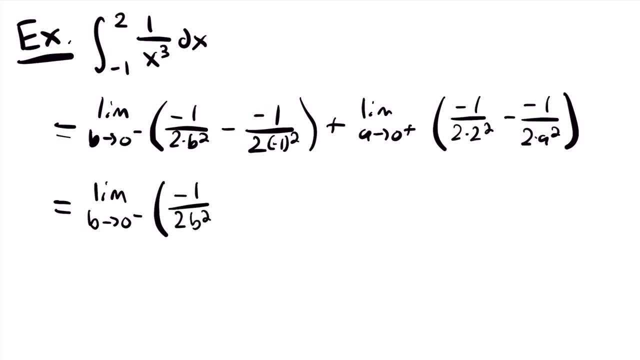 one divided by two b squared, Then these two negatives will cancel out. So we have plus one divided by two times b squared, And then we'll add our second limit as a approaches zero from the right of negative one divided by two times negative one squared. 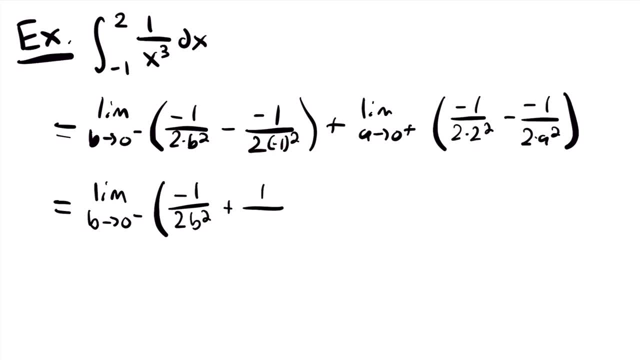 Negative one squared is just positive one. so one times two is two, So we have one half. Then, plus the limit as a approaches zero from the right of negative one divided by two times two squared, Two squared is four times two is eight. so we have negative one eighth. 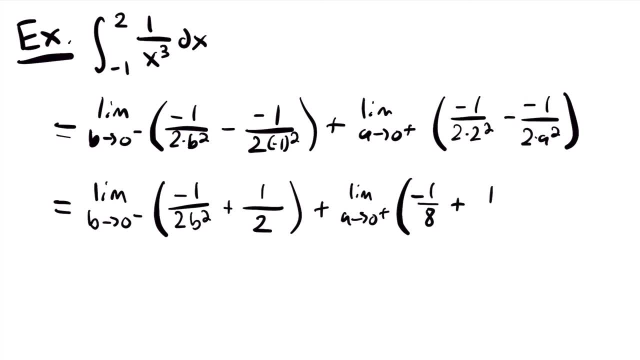 And then these two negatives will cancel out. So we will have plus one divided by two times a squared Okay, And so now we're ready to evaluate the limit, Okay, of each of these expressions, but we're going to need a little bit more room to do that. 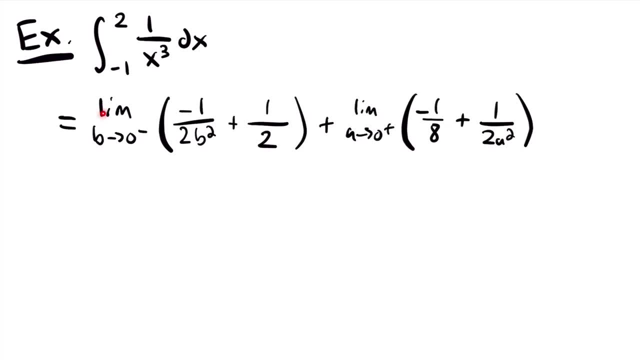 So let me clean up my work here. first, Let's start with this limit. we have the limit as b approaches zero from the left of negative one divided by two b squared, And so what happens to this expression as b approaches zero? Well, if we plug in zero, we have two. 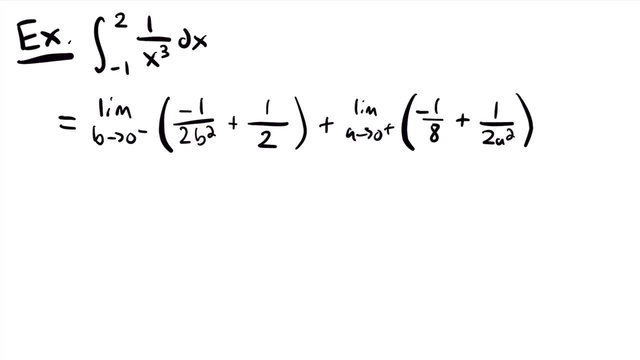 times zero squared, And so you have zero in the denominator, And so that's no good. So we have to plug in values close to zero from the left, And so if we're taking a look at negative one divided by two times b squared, let's see what happens to this expression. 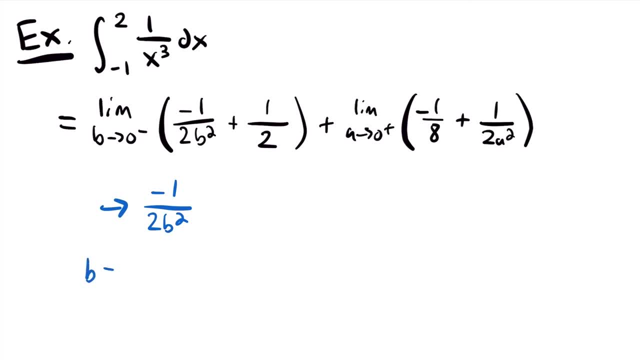 as b approaches zero from the left. So I'll start by letting b equal negative 0.1.. If we do that, this expression will become negative 50.. If we let b equal negative 0.01, which is a value even closer to zero from the left side. 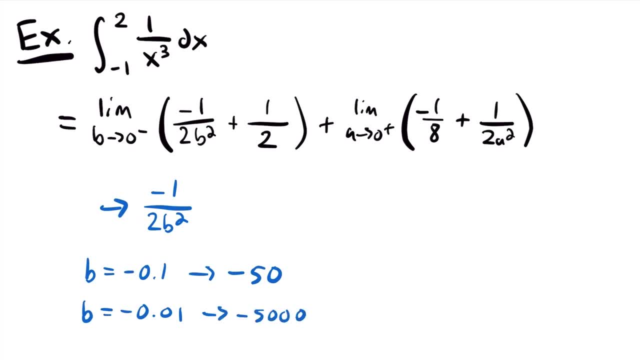 then this expression will become negative 5000.. And so as we pick values of B that are closer and closer to zero from the left side, we find that this expression becomes a larger and larger negative value, And so we can say that the limit of that expression is negative. 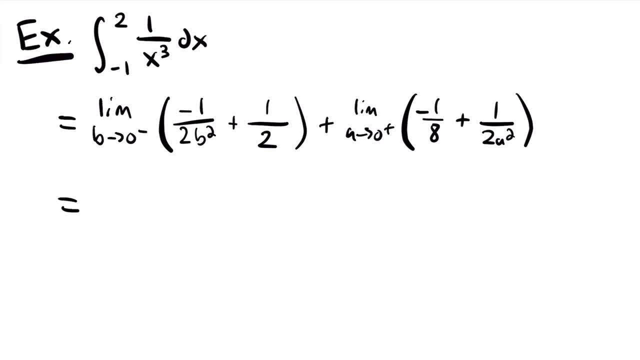 infinity. So erase this will have that this is equal to negative infinity plus the limit of one half, which is just going to be one half. But one half plus negative infinity is still negative 0.01.. All right, here I'll take a look at this next expression And we'll 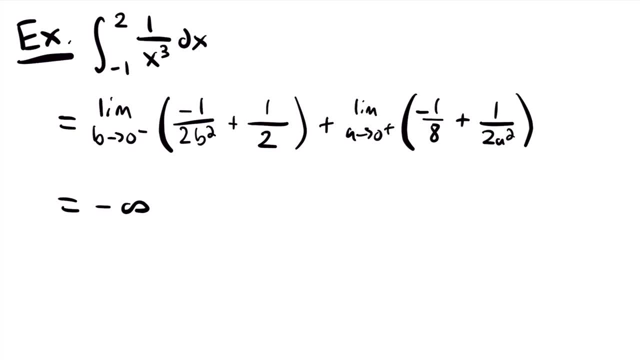 see what we end up with here when we plug in this expression at the end we'll know how to infinity. So I'm just going to erase that. We don't even need to have that, And then this will be added to this limit. Now the limit as a approaches zero from the right of negative one. 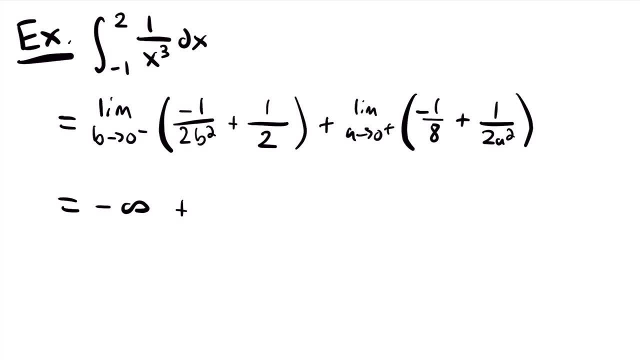 eighth is negative one eighth, And so we could write that, But for the same reason that I erased one half negative one eighth plus negative infinity is still negative infinity, And so we don't need to worry about that value. But what about this last term? We have one divided by two. 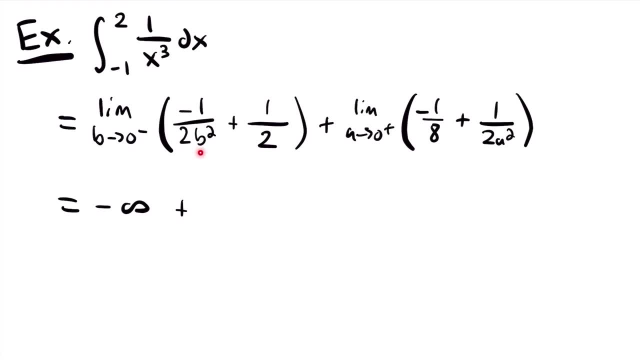 a squared. Well, this is very similar to negative one divided by two b squared, except it's positive And we're looking at what happens to a as it approaches zero from the right side instead. Okay, so we're going to have to plug in values close to zero from the right side again. 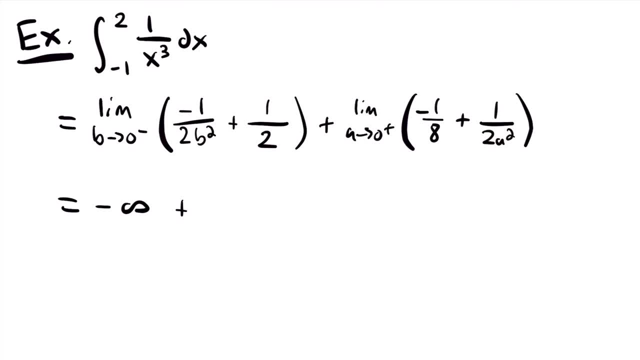 because plugging in zero gives us an undefined value. So if we're working with one divided by two, a squared, and we let a be equal to 0.1, that will give us a value of positive 50.. If we let a, be equal to zero, we get a positive 50. And if we let a be equal to 0.1, that will give us a value of positive 50.. If we let a be equal to 0.1, that will give us a value of positive 50. If we let a be. 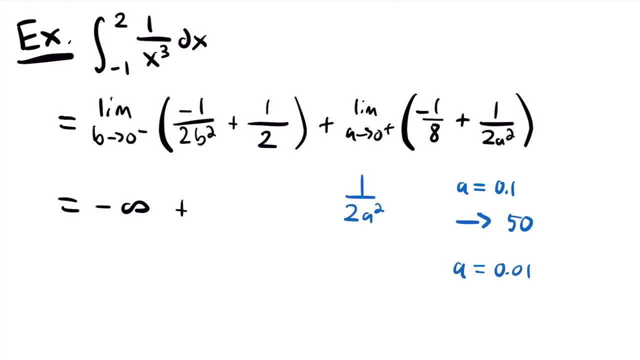 equal to 0.01, which is even closer to zero from the right side, then that expression will become 5000.. Alright, so that's what you get when you plug each of these values into this expression. So, as you can see, as we pick a value of a closer and closer to zero from the right side,